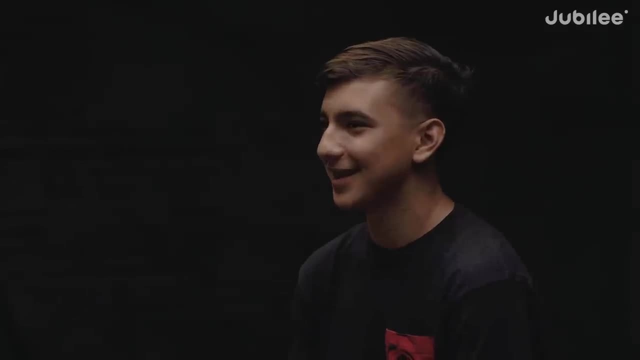 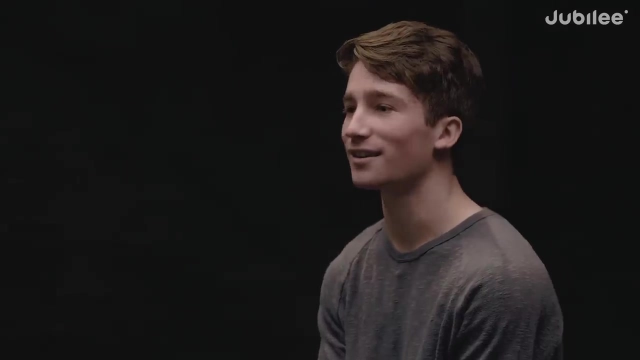 Well, first comes to mind is like preppy doesn't really go outside of like their house kind of. I got a 4.2 GPA Exiting high school. I worked my ass off to get straight A. I want to get a nursing degree, But if I want to, I'll go to medical school and become a neurosurgeon. 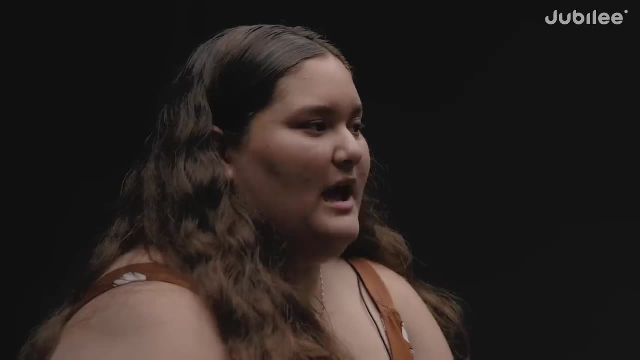 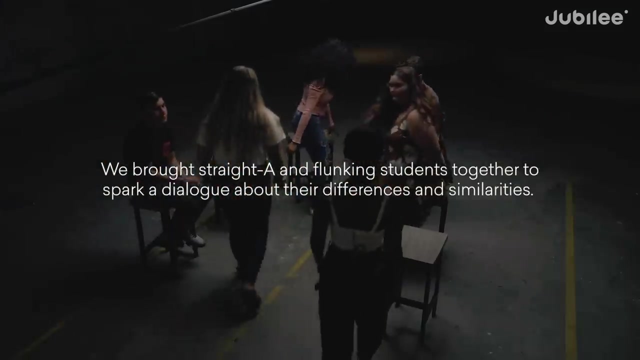 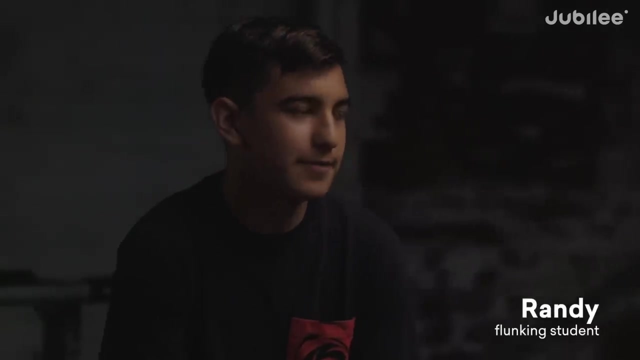 Um, of course I'm disappointed in myself. better Let myself fail, but I'm not gonna beat myself up for one-letter grade. I'm Randy, I'm 15 and I'm going into my sophomore year. I'm grace, I'm 16.. I'm going into my junior year, Hi. 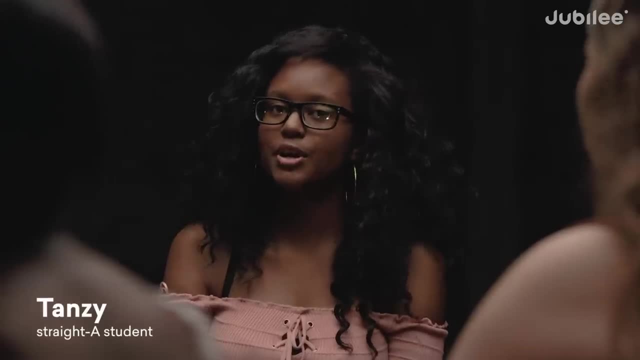 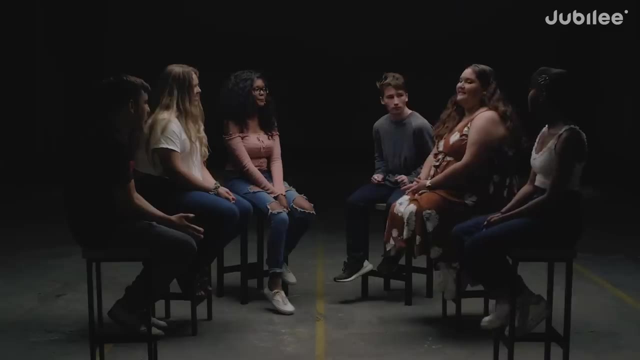 I'm Tansey, I'm 16 and I'm going into my senior year of high school, and I'm also a freshman in college. I'm Cooper, I'm 18 and I just graduated senior year. I'm Nadia, I'm 15 and I'm going into my sophomore year of high school. 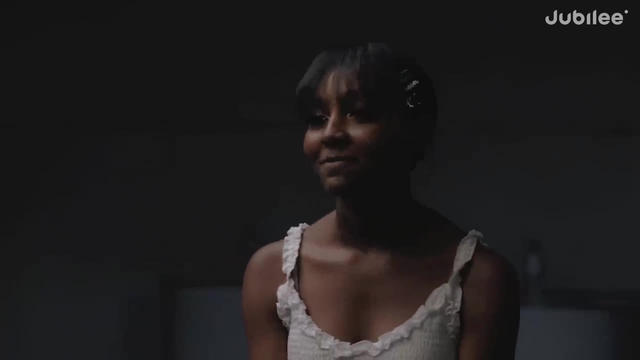 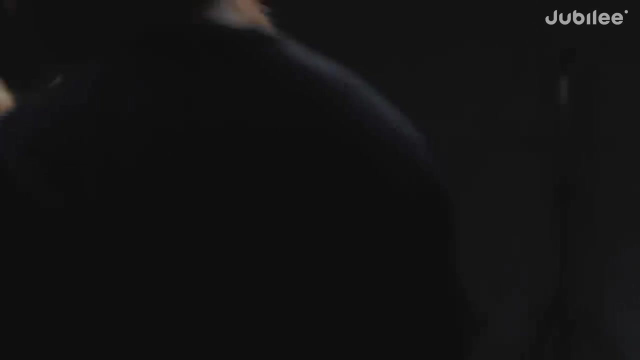 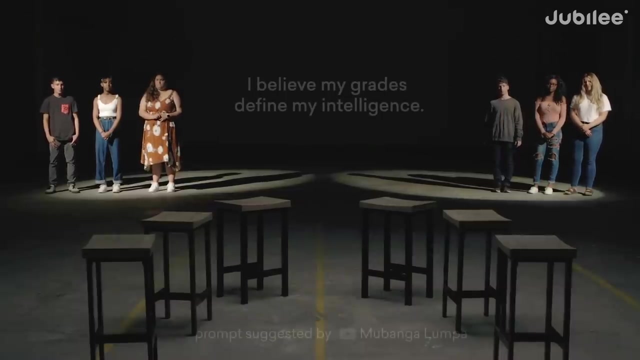 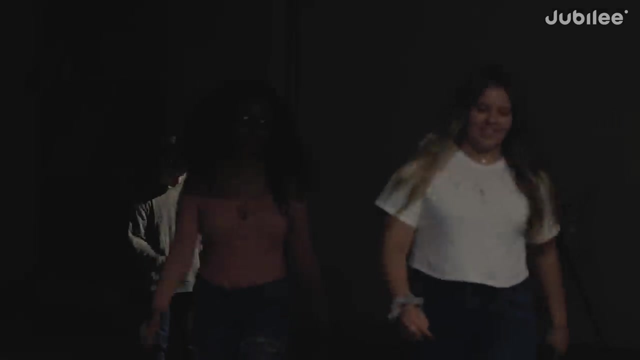 I'm Naima and I'm going to my sophomore year. Can I get my flunking students on the left and my straight students on the right? I believe my grades define my intelligence. I definitely think my grades define, like, how smart I am. 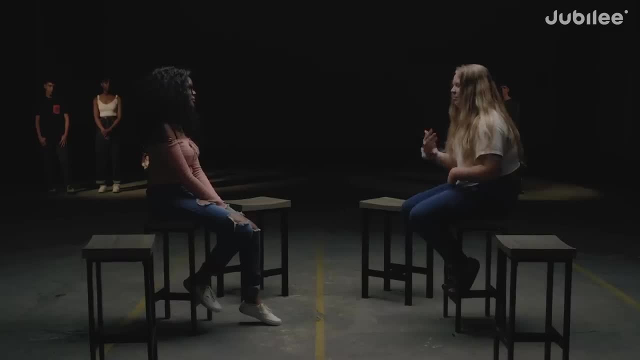 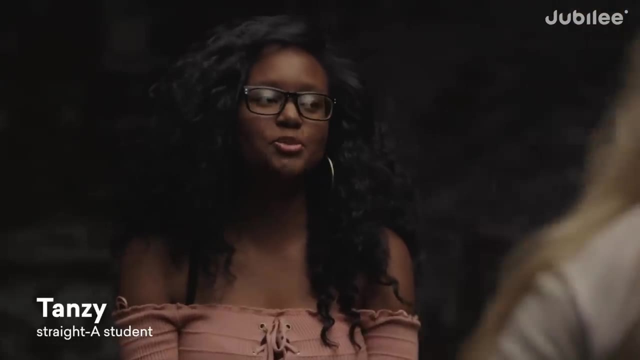 Like that's the biggest like security point I have, like in like as a person and I've just always been smart and like I always want people to think I'm smart. Yeah, I believe like that's really true for me. I believe like some subjects will enable you to show your intellect in some way, shape or form. 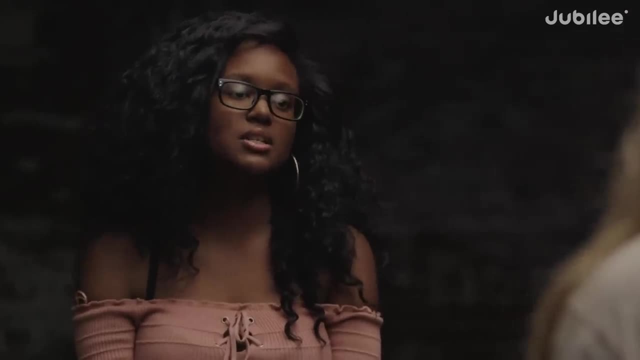 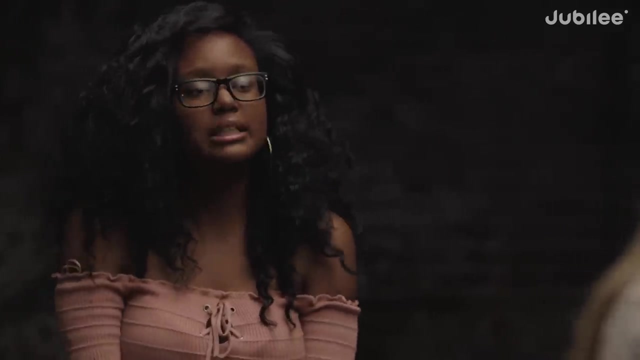 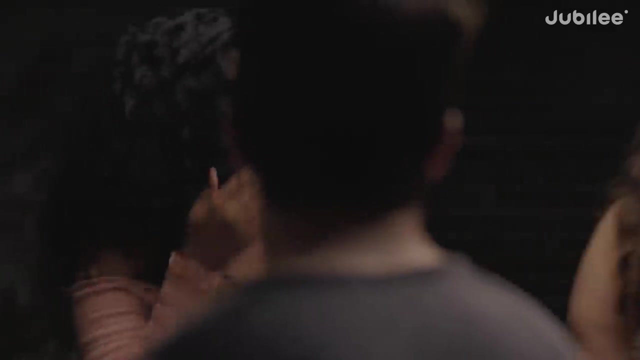 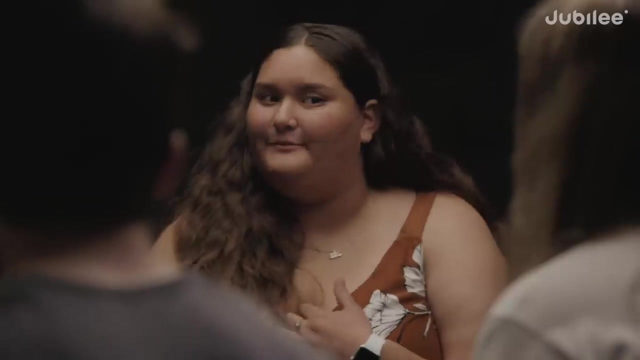 like math, but I do think that grades can show someone's intellect, whether it's, you know, understanding a concept or enabling themselves to you know grasp a subject. I didn't step up because I don't believe, because I'm not comprehending the concept of geometry, or algebra or poetry. that's not make me dumb. 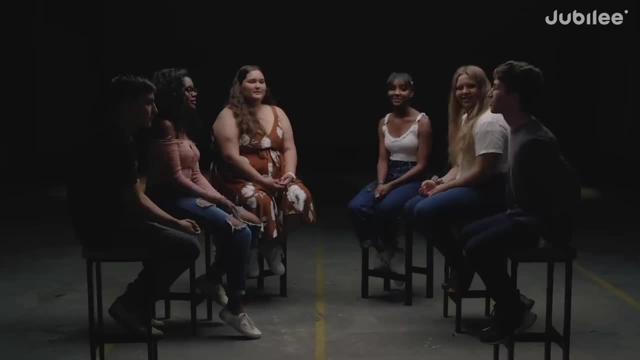 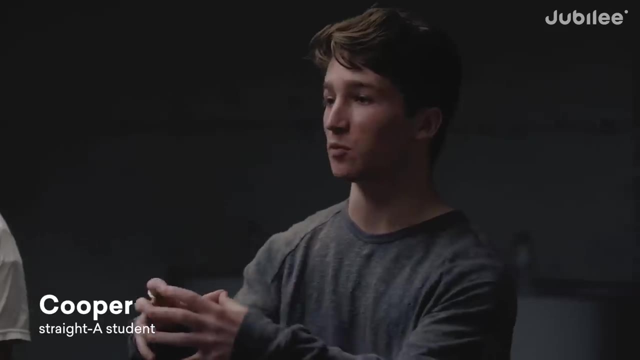 or that doesn't not make me less smart of a person. Yeah, I think also. people have different styles of learning and a lot of times schools try to put you in this mold of how they, how they want you to get a certain grade, and people aren't always made for that mold. 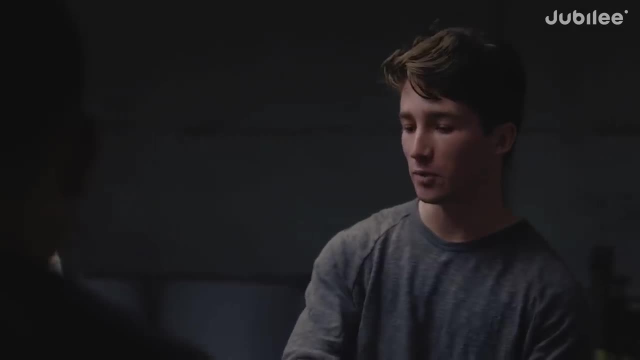 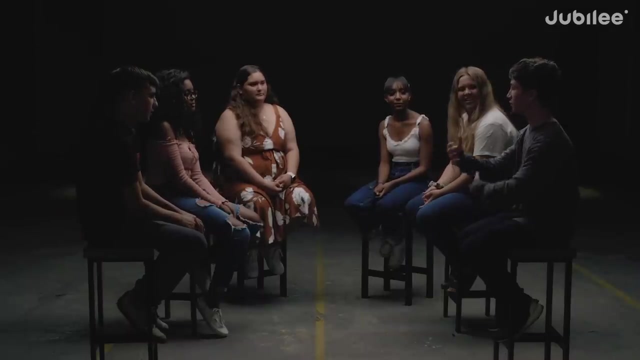 and it's really important that I think schools take into account that not all people are willing to learn by reading a book, and so to measure that based on a certain letter is, I just feel like so, like superficial. it's looking at it so one-sided. 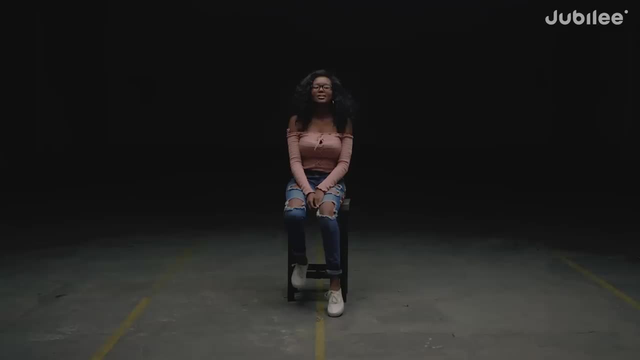 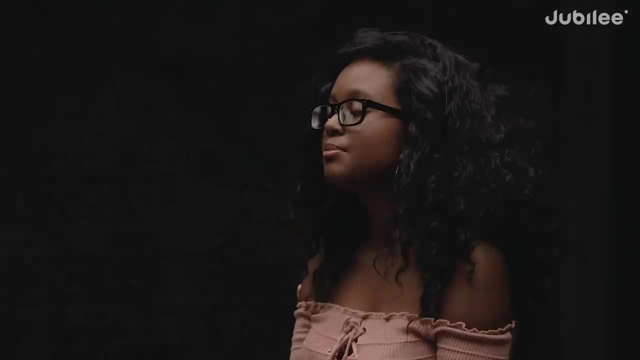 Are you proud of being a straight A student? I am, because it kind of like shows all my hard work and all that, because I come from like a family that really didn't have anything and being a straight A student allows me to pay homage to all their hard work, and so it makes me really proud to be able to. 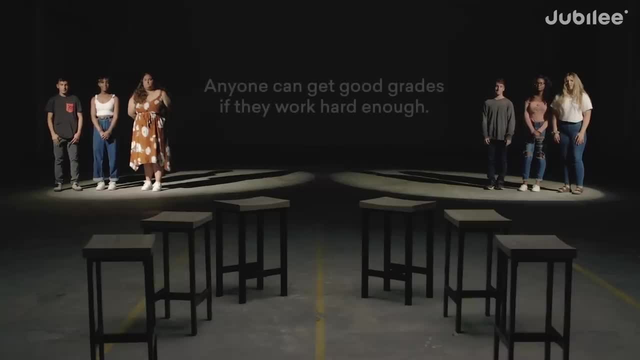 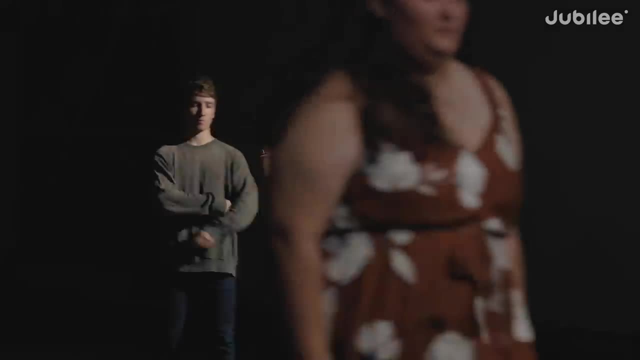 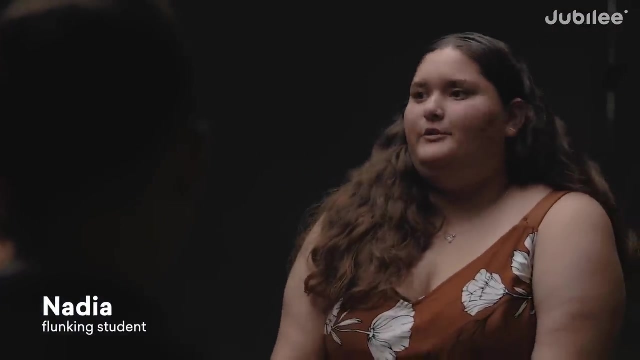 you know, honor them in some sort of way. Anyone can get good grades if they work hard enough, Of course, like if you try your hardest and if you do all your work, you do all your homework, you're going to push, you're going to get good grades, just because you're not comprehending it. 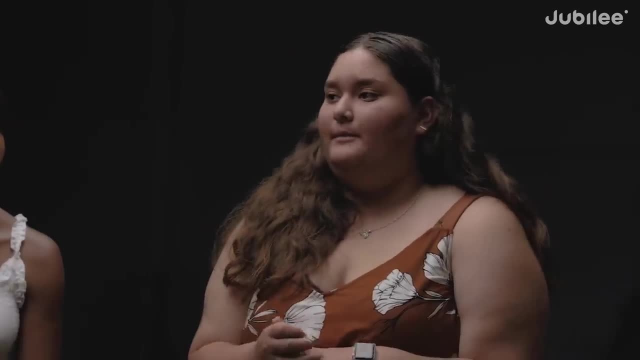 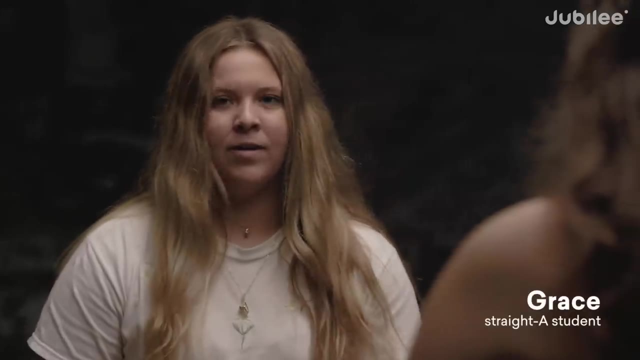 doesn't mean that you're not going to get the good grade. yeah, you might struggle, but with help and hard work you're going to get there eventually. So I definitely think there's two sides to hard work itself, because working hard that can mean like studying and like working super hard to better your own skills, but you can also 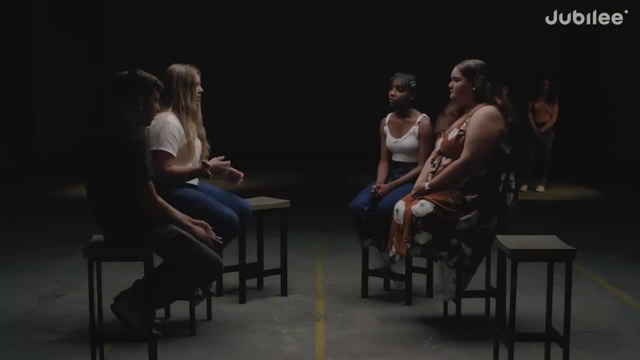 work super hard to cheat and work super hard to get answers to tests and work super hard in that manner. but at the end of the day, I also feel like if I work super hard, you're going to see what I see when you study. But if you study hard, you are going to notice that it's hard and that's not going to get you to where you are. 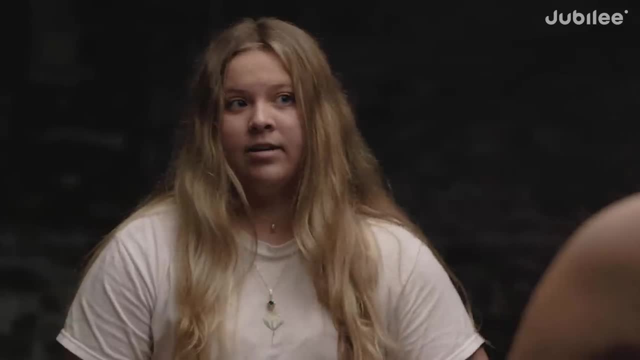 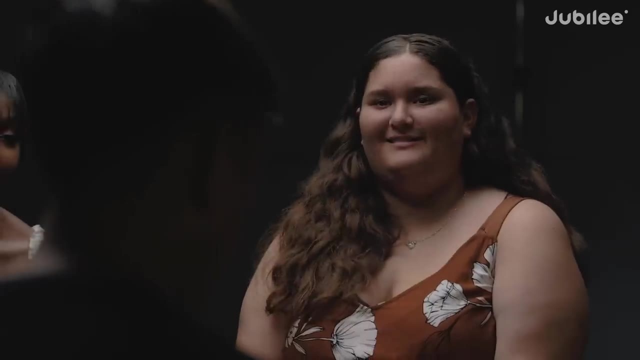 But at the end of the day it still might get you a good grade on either side. You guys think cheating is pretty common. Yes, definitely For the most part. a lot of people tend to cheat on tests, copy, homework And, depending on how the teacher might grade the grading system. 85% of your class grade could be homework. You cheat on all your homework assignments. You have a B right there. If you're the type of person where you can put your mind to something and never give up on it, you'll get that grade. 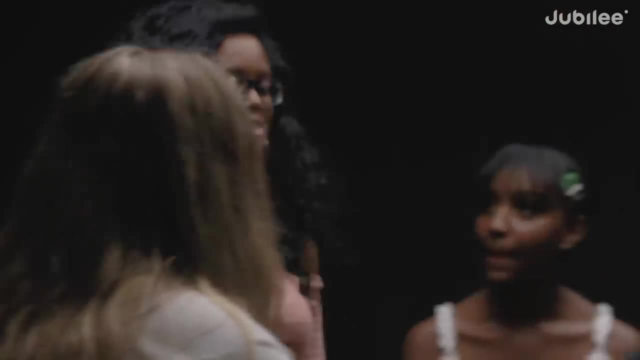 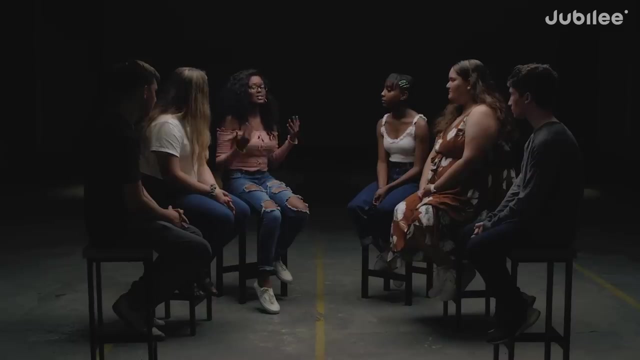 I've had a 7th grade teacher- my English teacher- and I tried my hardest in her class. Meanwhile I didn't know- innocent me- that she was full-blown racist, okay, So I was sitting there in that classroom working my hardest. 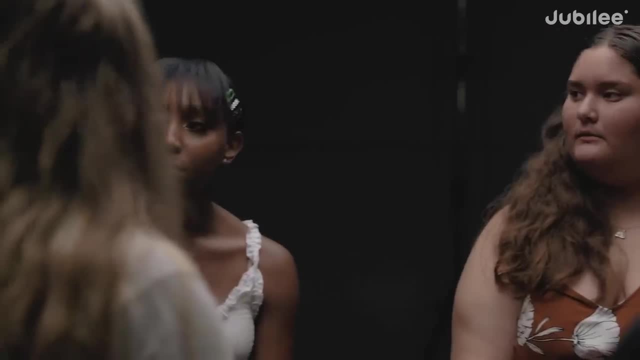 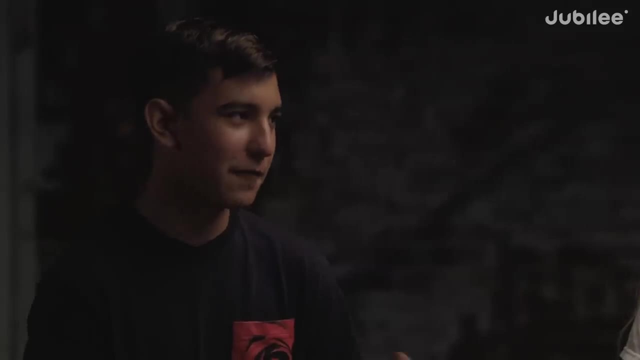 making C's, knowing I can make A's, and it put me down so much with my self-esteem. It also depends on your personal standpoint with the actual teacher themselves. Clearly, if you're provoking a teacher, you know like. 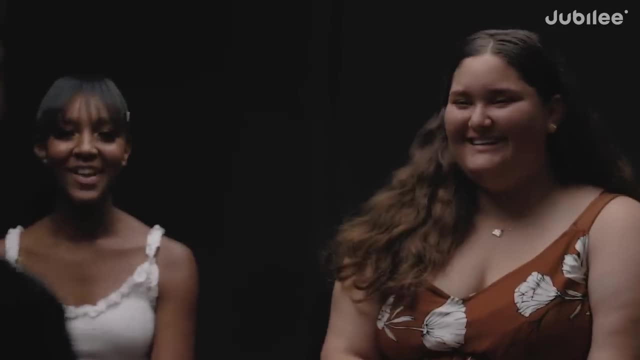 I do it all the time Like they're not going to like you, But like I've learned that That's a lesson in itself. that's like an experience. of learning is that you need to make friends with your teachers. 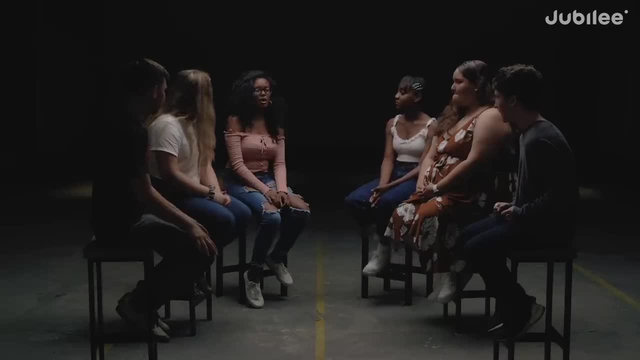 They'll want to give you a good grade if you're friends with them. There's some concepts and I'm going back to like personal, like experiences. In 8th grade I couldn't get exponents to save my life. 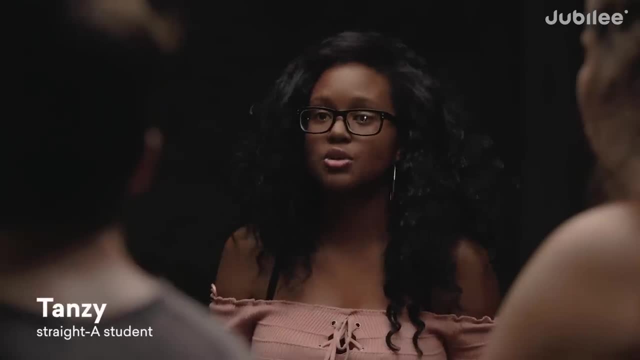 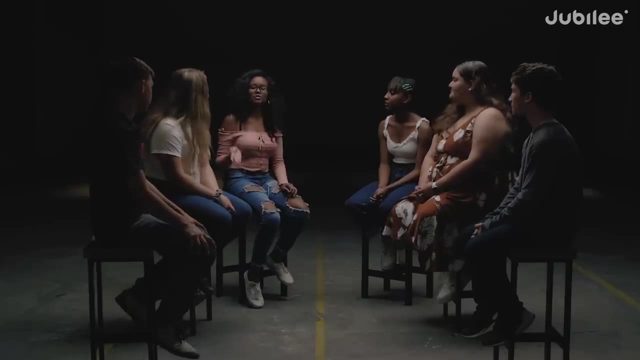 I went to tutoring, You know. I stayed after school, had parent-teacher conferences because they thought I was being a bad kid and not studying. They thought I was failing on purpose. It took me my freshman year of high school to realize like, oh my God, this is so simple. 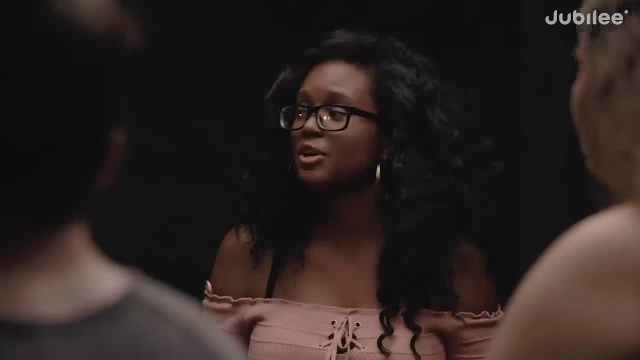 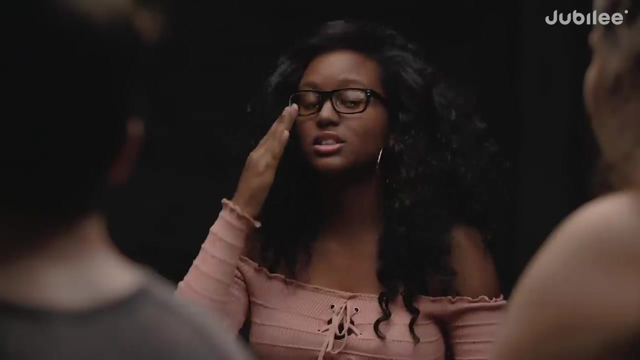 There's certain learning blocks that you can face within yourself. It doesn't necessarily have to be teachers, It doesn't necessarily have to be like social problems. It could be all in your head And if it takes that one roadblock, it will like stop everything. 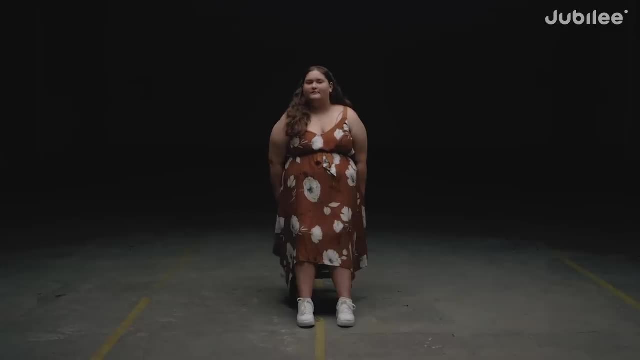 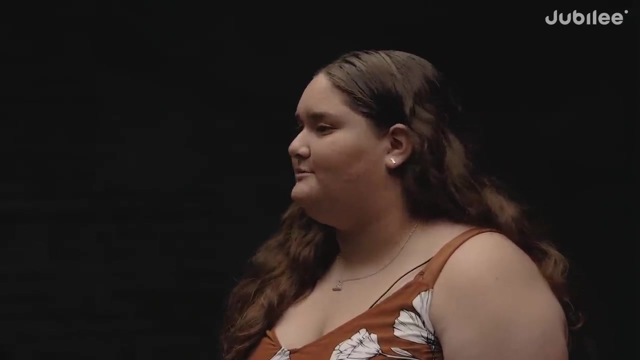 Are you self-conscious of your grades? No, I'm not self-conscious, because I know there's a lot more students that are in my same boat who aren't dumb. They just have trouble comprehending certain subjects. I can relate. I can relate to the other side. 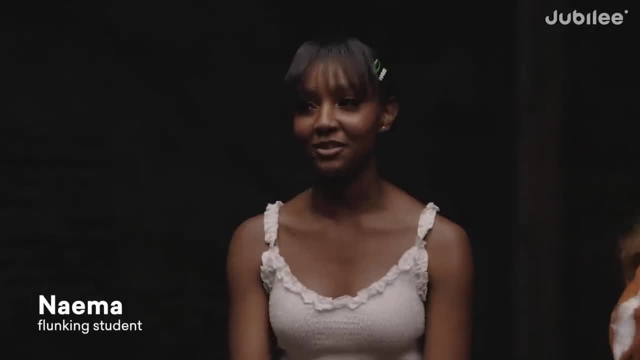 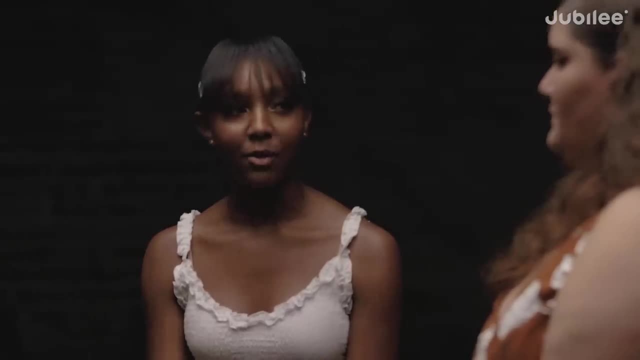 So I've never gotten straight A's ever Like. I've never been like in the top of my class. I've always been struggling or I've always been just in the middle. Just yeah, I mean ever since I was younger. 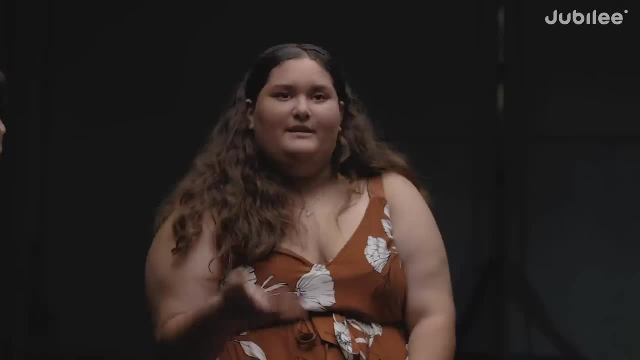 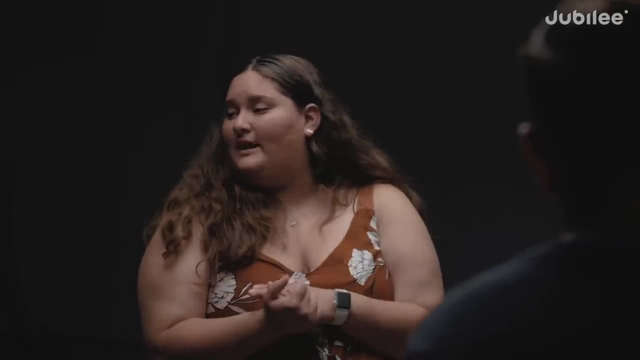 I was always in an extra class to like help me with my work. Like my elementary school, they had a gifted program. I was never in the gifted program. There are some ways I can relate Like I still am working hard. 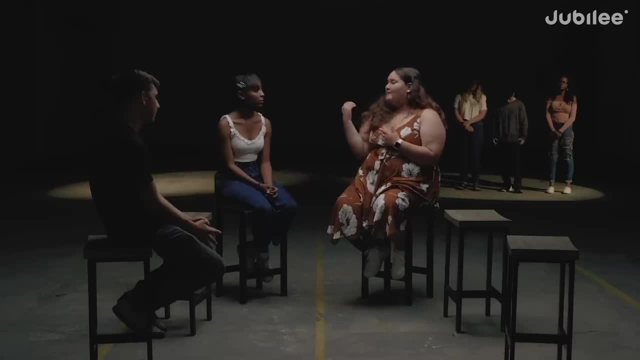 I still am making sure that I get the best grades that I possibly can, But I'm not like them. I don't stay up till 3 in the morning to study. I don't stay up till 3 in the morning to do a project. 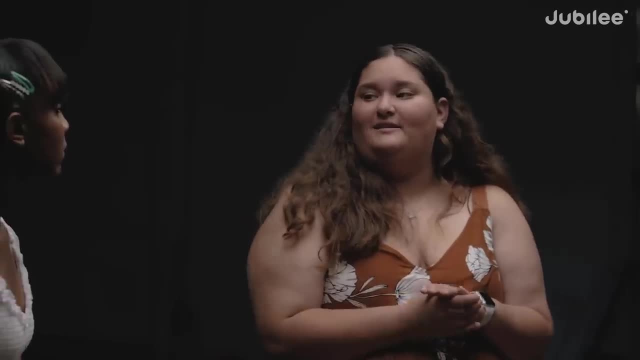 I'll stay up till probably like 1, and I'm- like you know what I'm done- Like I need my rest because the next day I'm going to go to school and be all tired and be all frustrated. 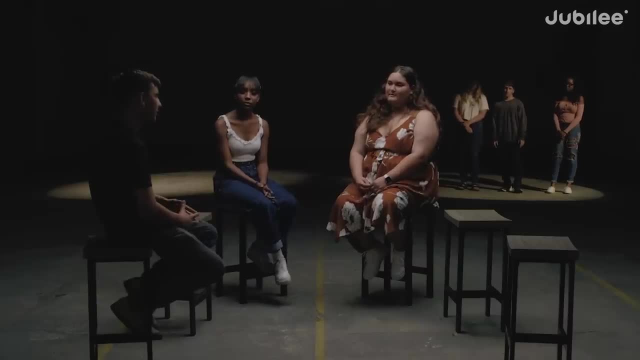 And then it's just too much. so, Like being like the idea of being a straight-A student I can't relate to. I'm always wanting to go out and like I have an essay due, or like there's a paper that I have. 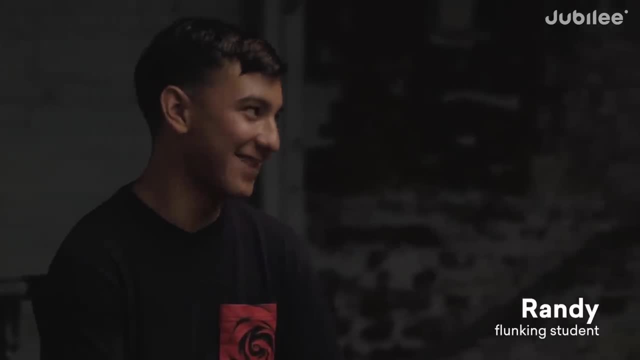 and you know there's a paper but there's a skateboard. I'm going to hop on that skateboard Like I'm out, Like the fun I have, just hanging out with friends and just like doing whatever we want whenever we want. 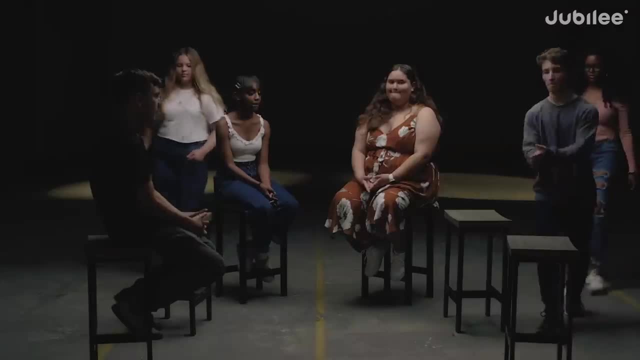 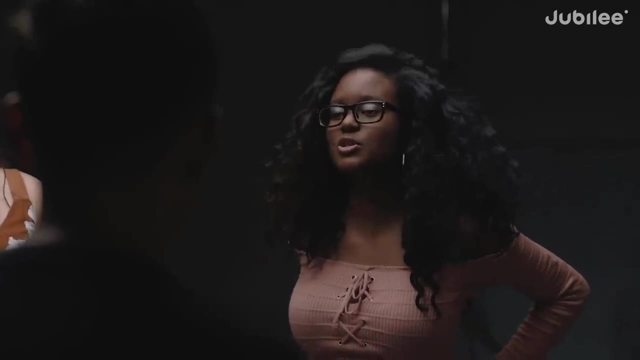 it's just so much better than like: wow, I just got an A, Like you know. Okay, so I can definitely relate to the idea of being a flunking student, because I feel like there's two types. There's one type that doesn't choose to do the work. 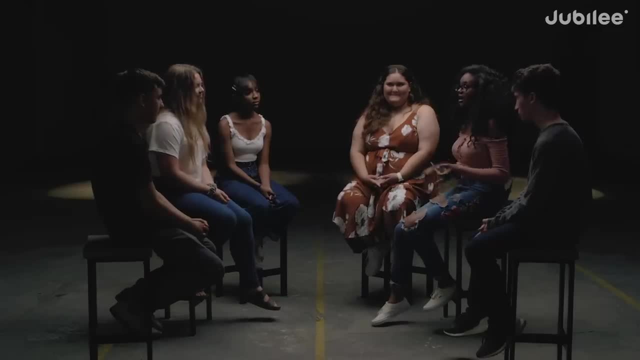 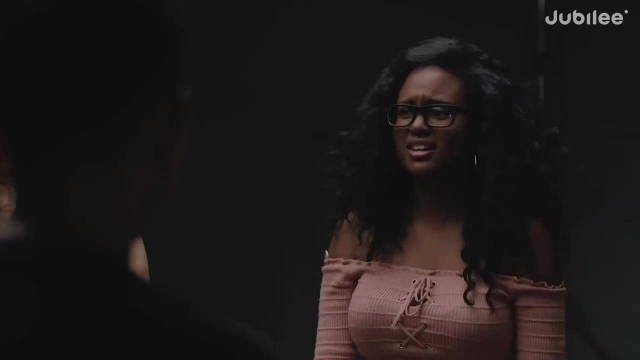 and then there's the other type of where I cannot understand this. I need help, and I relate to both, because there's some times where, like I've gotten a grade on a test, like I failed it, and there's times like I'm not going to retake that. 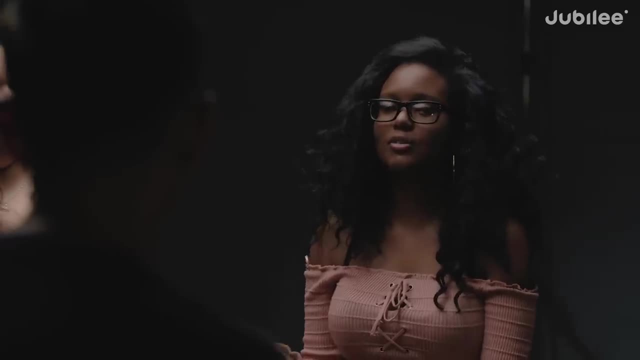 Like that's too hard, Why would I waste my time? And then there's times where I'm like, oh, my freaking God, like I cannot understand this for the life of me. I need help. which is fine, because not everyone's going to get things like 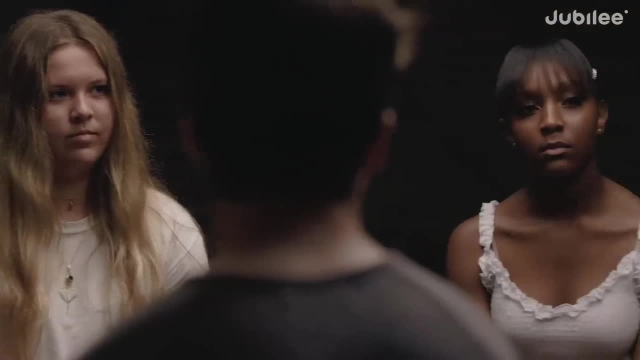 a drop of a dime. you know There's some people that do, There's some people that don't. I can 100% relate to you guys because I know what it feels like to be sitting at a desk at 11 at night. 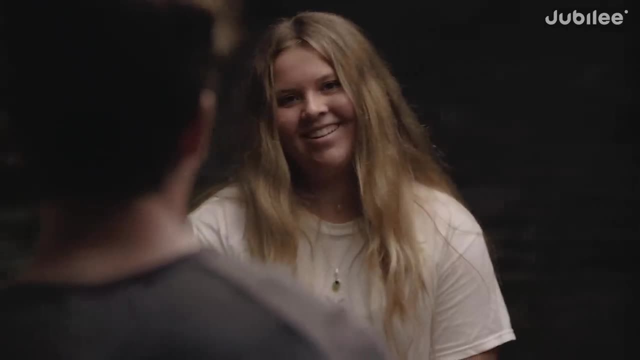 and wondering how in the hell am I going to finish this? And luckily I've been able to push through, but I can see how someone couldn't. I fully relate with all of you guys because at some points I've questioned like 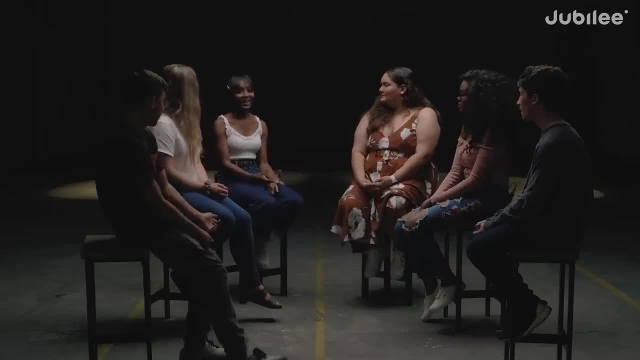 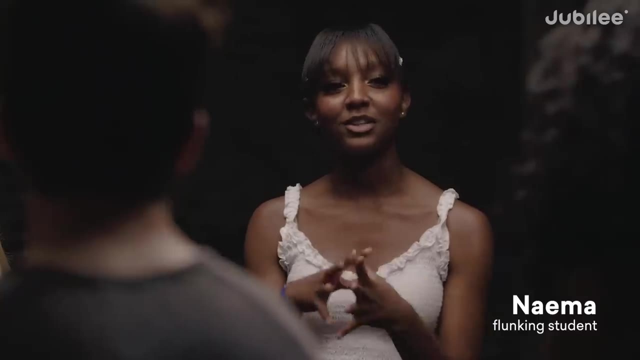 maybe I should just go in and not study for the test. Yeah, I don't. I feel that, like just some of you guys don't like, relate to as much as you think being a flunking student like flunking a lot. 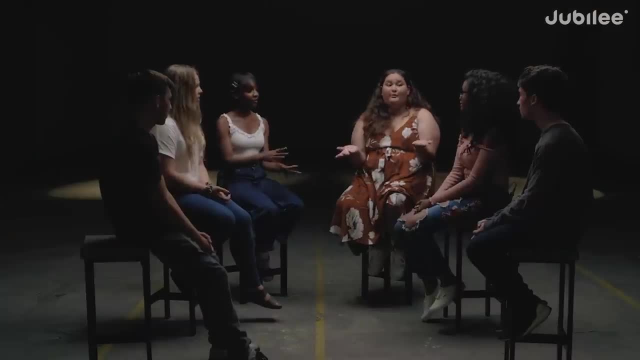 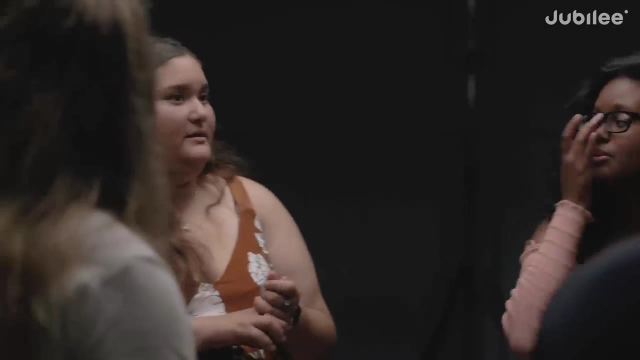 not just one class and you guys still have 4.0s. I'm lucky if I pass the 2.0.. In a way I see you guys' point like when you say there's two types, but no matter what type of flunking student you are. 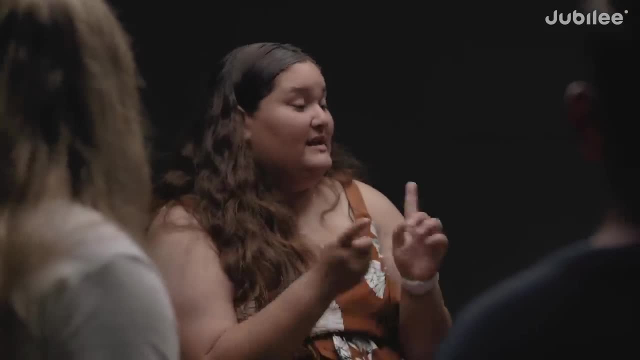 you are always going to be characterized with the stereotypes that a flunking student is not smart. they just don't do their work. they're lazy. I'm not going to say that. I'm an F student and I'm proud of it. 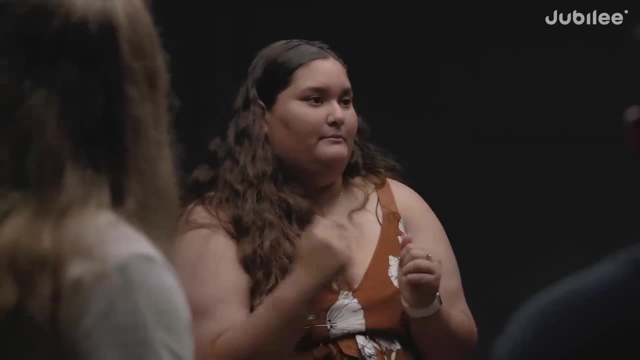 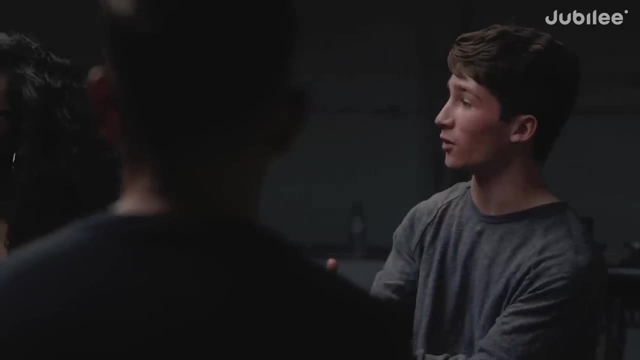 Of course I'm not proud about being an F student, but I'm not going to push myself down because I'm an F student. You're right. I can't relate to that idea of being a flunking student and having those eyeballs on you. 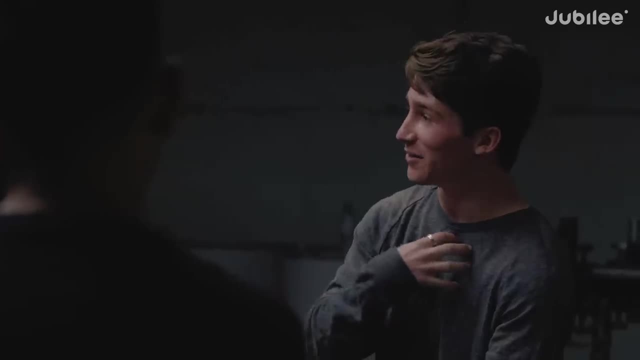 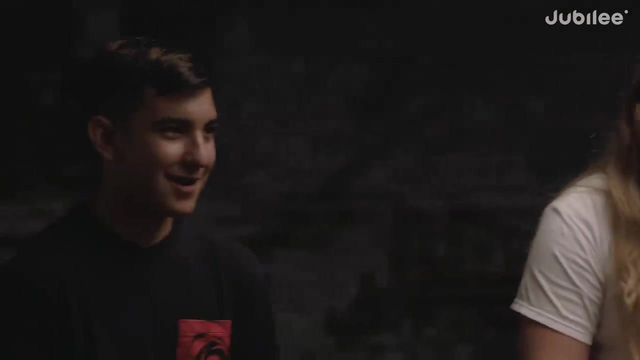 in a certain way, and I wish that I could, because I want to understand what that's like. It's the same with you guys aside. Yeah, at the same time, you guys have the nerd stereotype. You know what I mean. 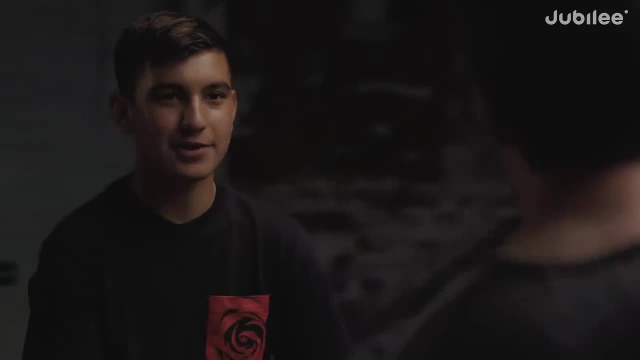 You could walk up to somebody who's one of us and we don't know you and you'd be like, yeah, I'm a flunking student. We're like: oh, so you sit in your room all day. You don't walk out of your room, huh. 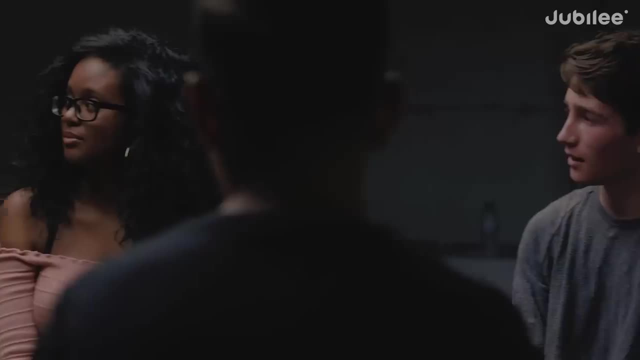 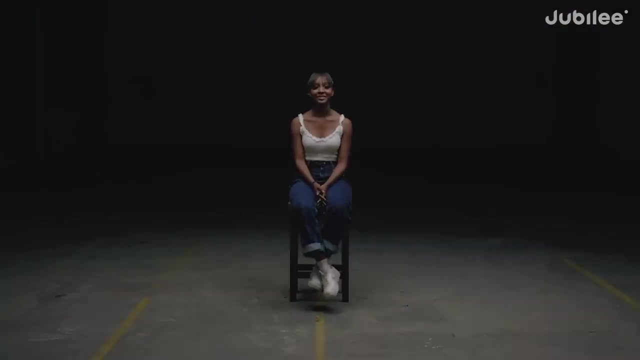 So, no matter what, there's always stereotypes. You can be completely different, but you're still going to be characterized as that certain stereotype. I do like school, yeah. Are there other things happening in your life that distract you from school? Yeah, a lot of stuff at home. 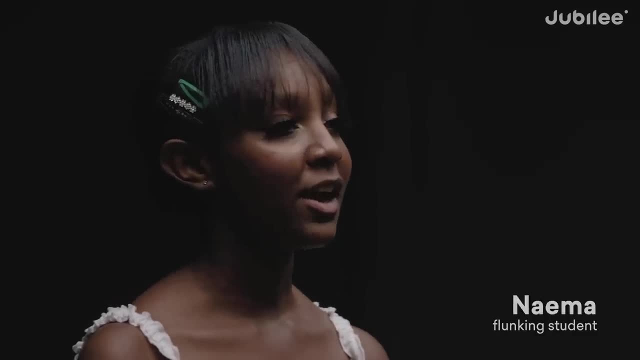 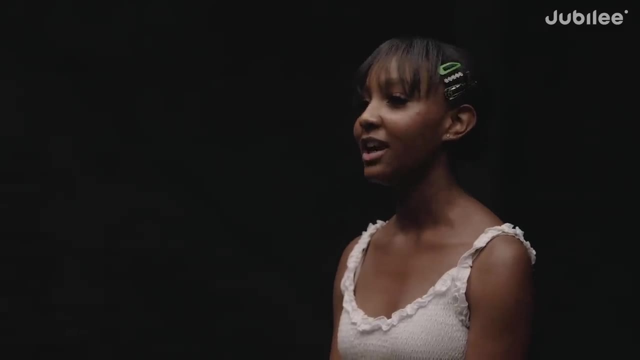 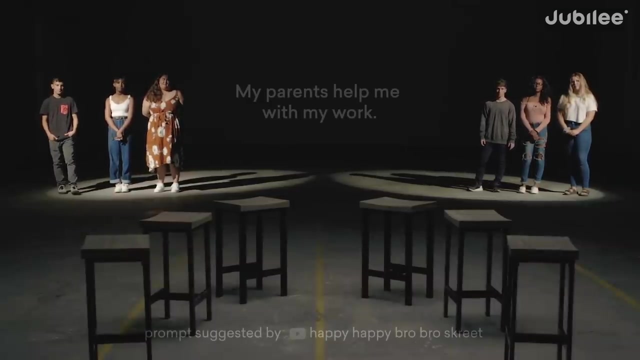 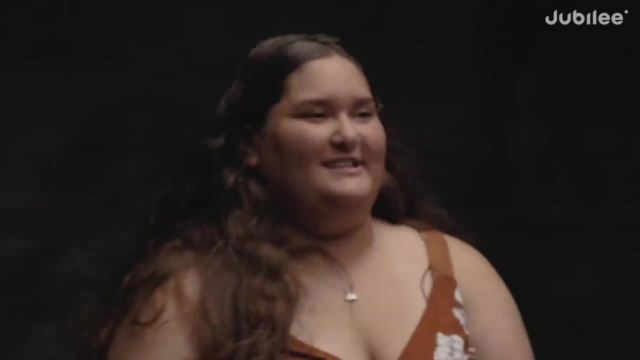 I struggled with my grandma dying and my parents splitting up and all that isn't good for my mental health, especially when I'm struggling with certain subjects and certain topics and tests and people. My parents helped me with my work. I won't say my mom helped me with my English work. 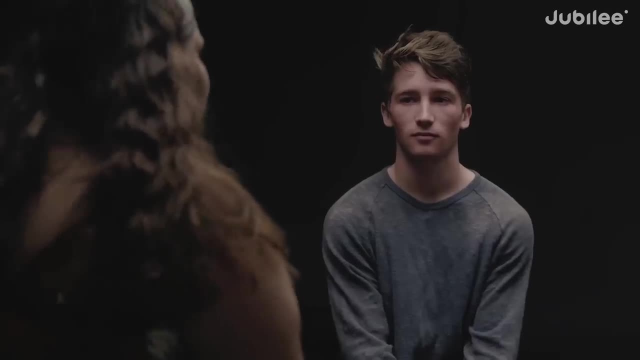 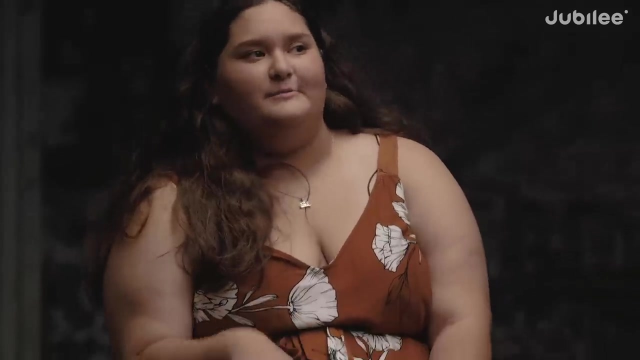 my math, my science. When I was doing theater, she would help me memorize my lines. She would help me write the essays to certain directors of the show. She pushes me to do it myself, which I'm glad about, but there are some times where I'm like. 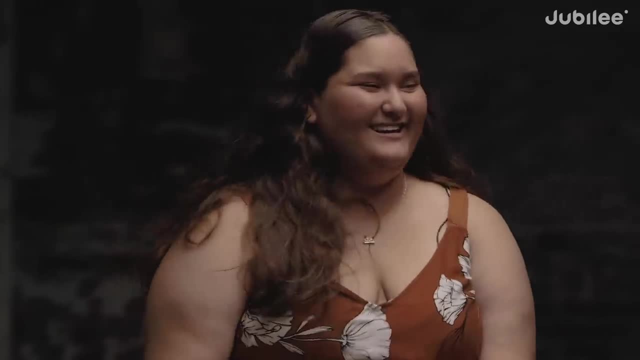 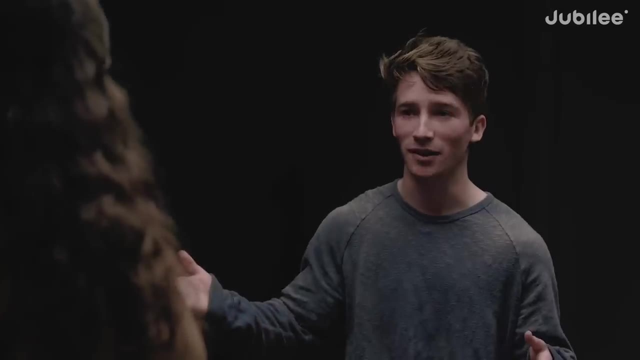 can you help me? And she's like I don't know it either. I'm like, okay, that's fine. My parents don't write my essays for me. My dad, he, dropped out of college. It's not like he's going to be helping me. 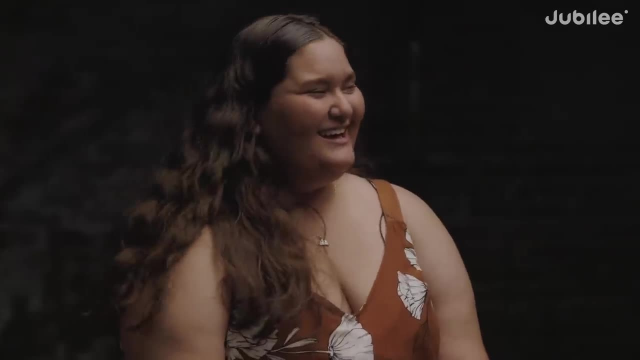 with my AP stats homework. Mom didn't even go to college, Yeah, But you know it's like he will. I think they help me do my work in the sense of like they keep me diligent. They are, in a sense, like instilling me. 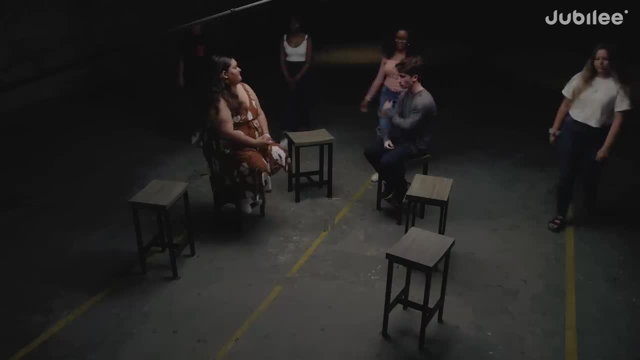 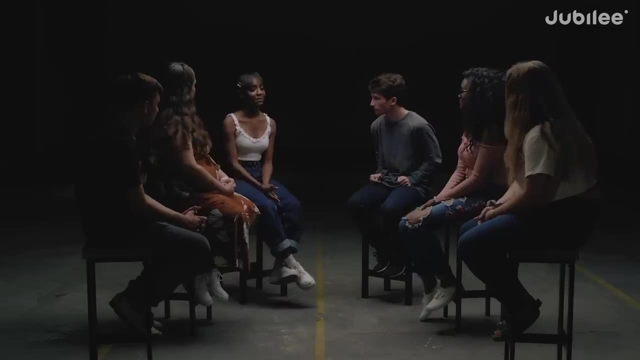 with the right qualities to write those essays. I feel like my mom looks at my paper and she's like girl, this is that new math? Like I can't do math. Same Like my mom, she can't help me really. 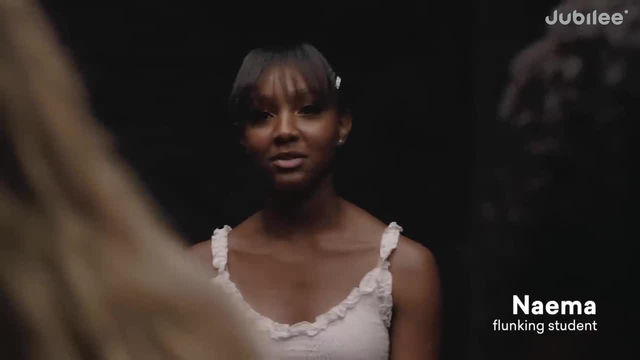 and neither can my dad. so Because when I get back from school, my mom's leaving to go to work. My dad works all day, and when he comes back home he's tired, And then I have to take care of my little sister. 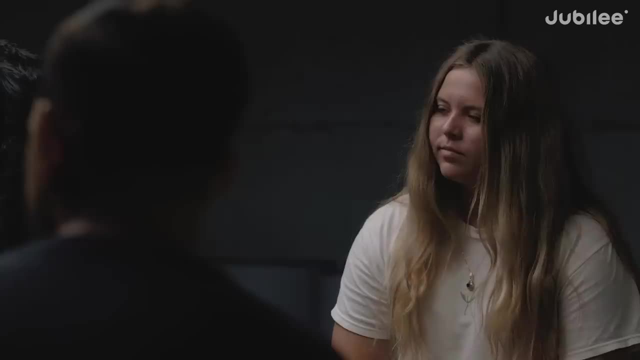 Even when my mom comes back. she comes back at like 2 in the morning and she still sees me up. I have to do that on my own, so With certain subjects my dad can definitely help me up. I take auto shop. 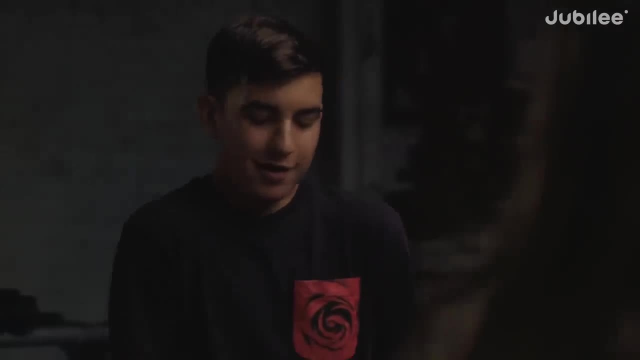 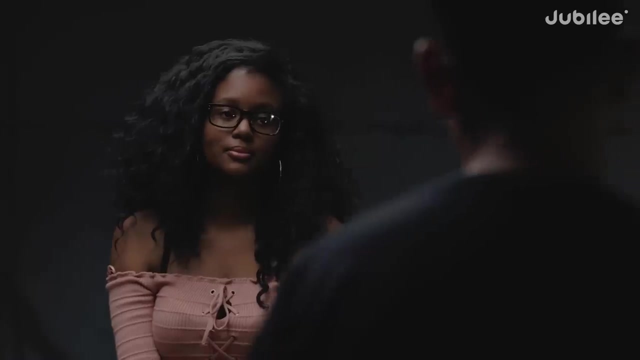 He's in automotive tech. Yeah Well, yeah, exactly. When it comes down to like actually doing it with normal subjects, he says to me like you need to figure it out because, at the end of the day, one day I'm not going to be there to help you at all. 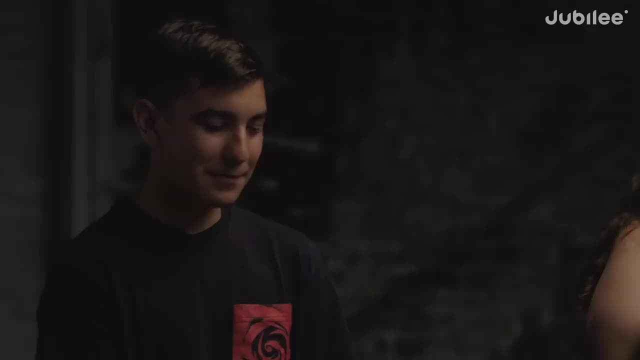 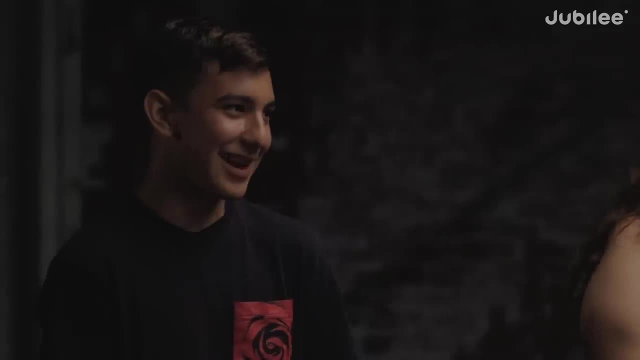 I'm going to put something down and like I'm going to turn it in. so when it comes out, don't be. Don't be surprised. like, What's your dream job? I want to be in automotive tech. 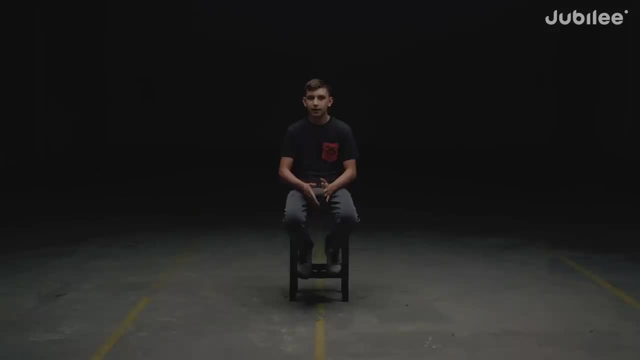 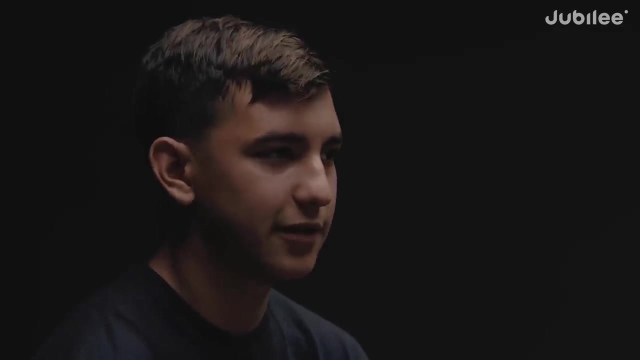 but then I would like to own my own business off of it. I know they like. they want to see me aspire to what I can be. It's hard to like, steer people to a different direction, to like, but this is what I would like to do. 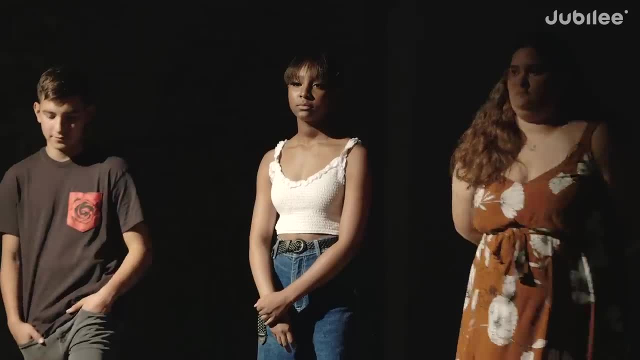 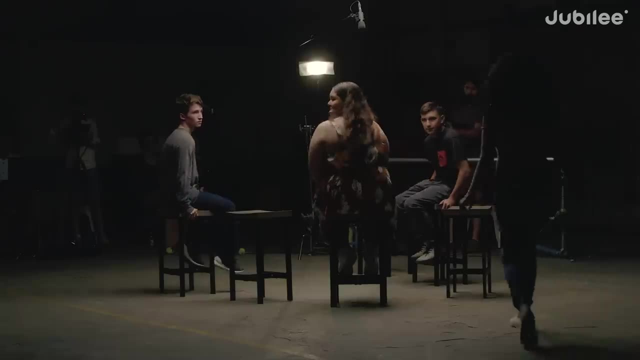 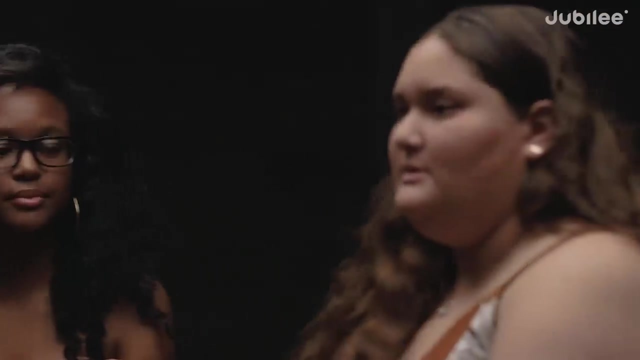 I deserve the grades I get. I do believe that I do deserve the grades I get, especially for the ones that I am failing, such as English. I'm not putting my 100% into the class. I'm probably giving like 50%, 75% if that. 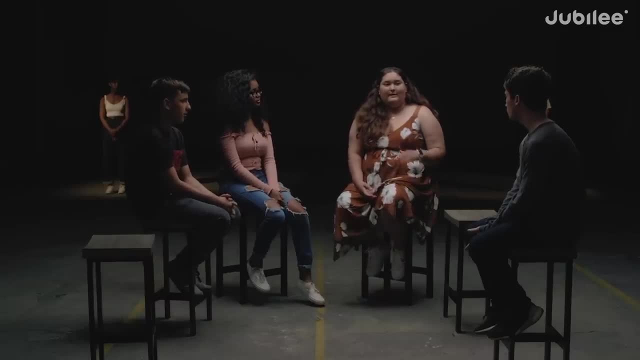 But for the grades that I am getting good at, like my film production class, I'm giving all. I'm focusing more on my extracurriculars than I am on my primary classes, which is my fault. It's nobody else's fault. 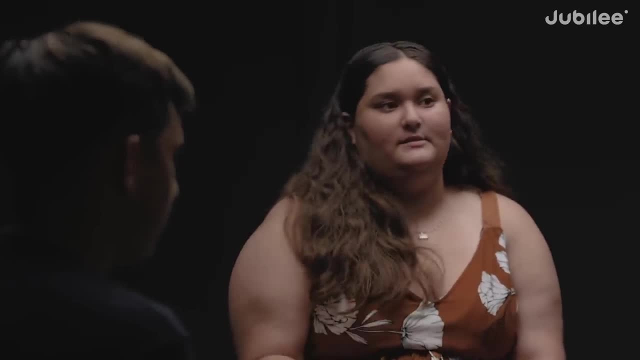 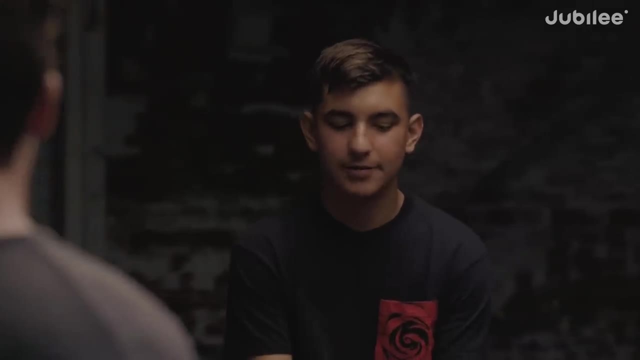 I am putting myself in a position where I'm letting myself flank these classes. I feel like I deserve the grade that I get, because I know I could get a better grade, but I choose not to because it's like the subject to me. 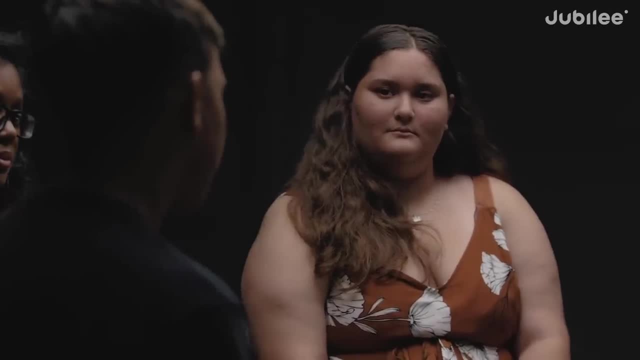 like it doesn't really click with me. Why am I going to sit here and put all of my effort to something that you want me to put, only to get like what you want to see? That's As long as I'm passing. 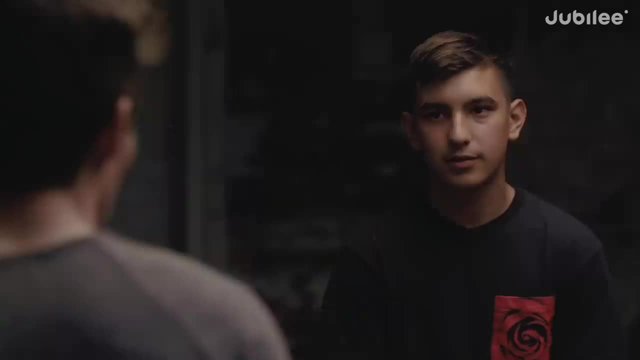 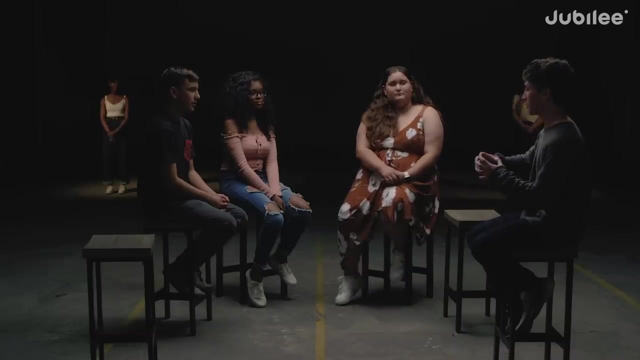 that's all I really care for. I mean, I've worked my ass off just so that I can get that good letter, And as much as I would have liked to just focus on film, I knew that in order for me to you know. 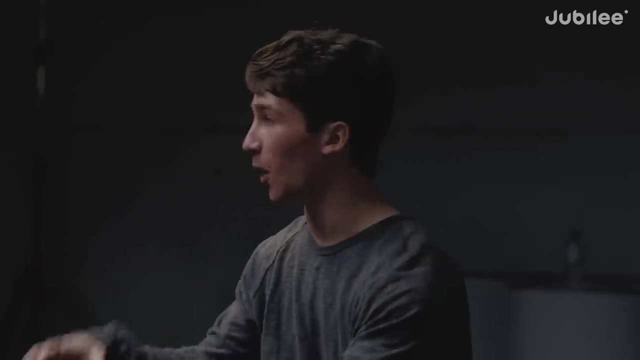 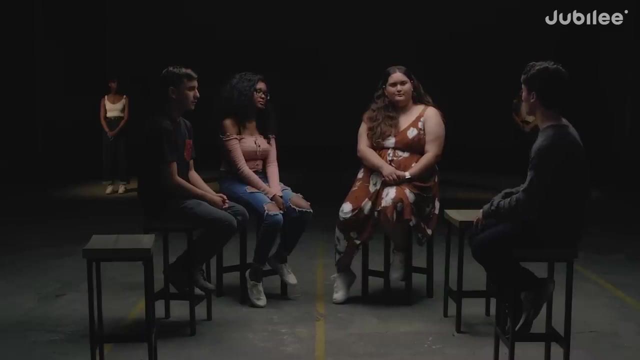 at least have self-esteem and feel like I was being successful. I had to do both And I don't know if, like that was the greatest thing to do. I don't know if that was the best decision, but I worked as hard as I possibly could. 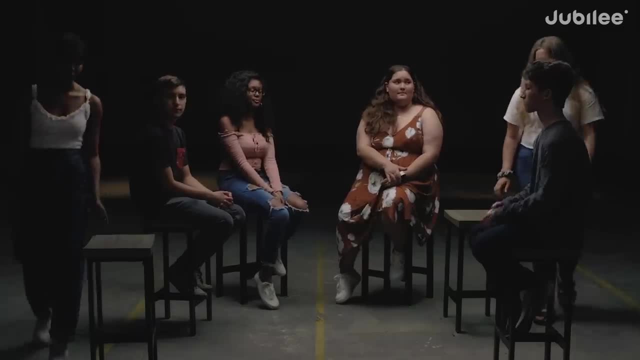 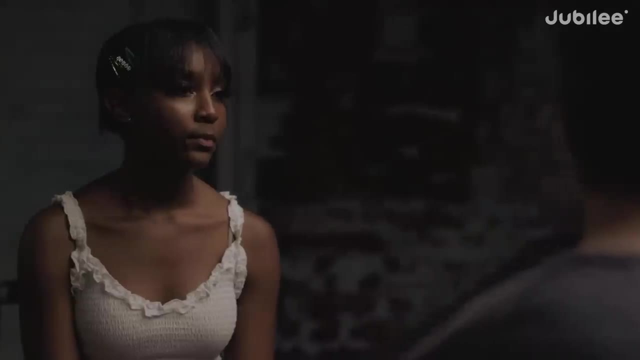 and I feel like I do deserve the grades that I got. I'm not ungrateful for the grades I get and I'm so happy with the grades I get. But, to be honest, sometimes I do just put like 50% of my work in. 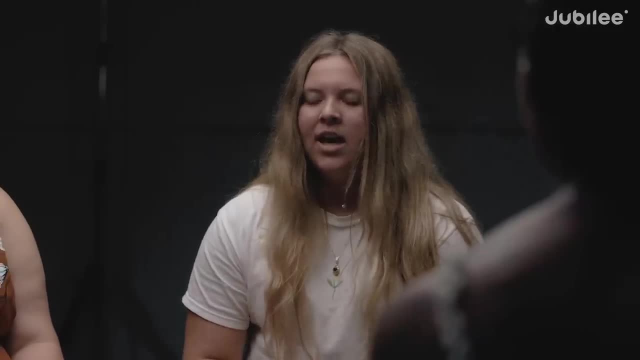 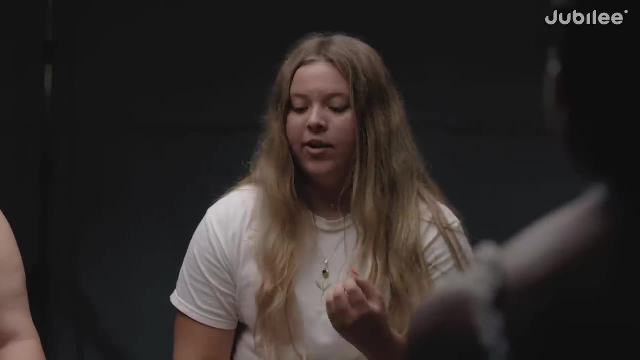 and I don't try my best But when I still do well on the project. I don't think I deserve that, because think about the kids who are like, working diligently on that project, trying to get a good grade, But just because I was able to finish it out. 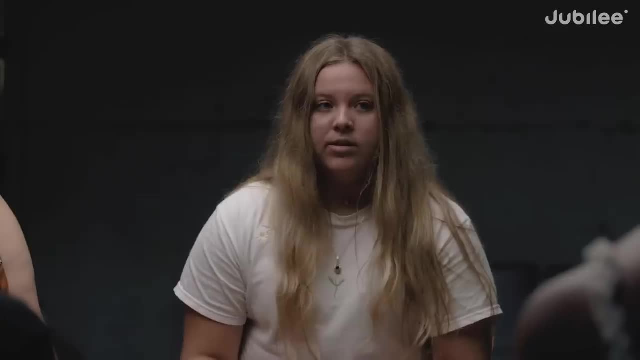 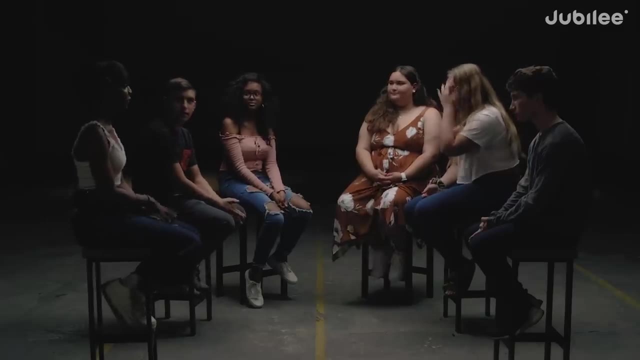 whip it out last minute, or my teacher likes me, or I'm a good student overall. I don't think that that's like a fair advantage to have. Yeah, I don't believe that I deserve the grades I get because I've had lots of group projects. 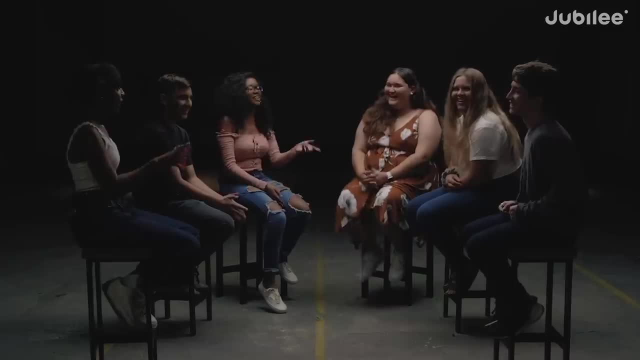 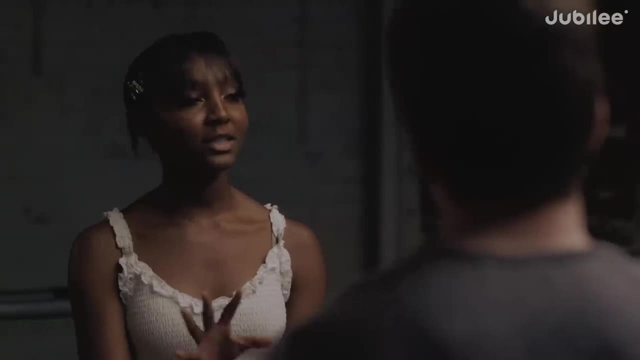 where it wasn't just me and it's always been other people. There was a time where I had a big slides project and I did most of the work but I only had like three slides for two other people to do. 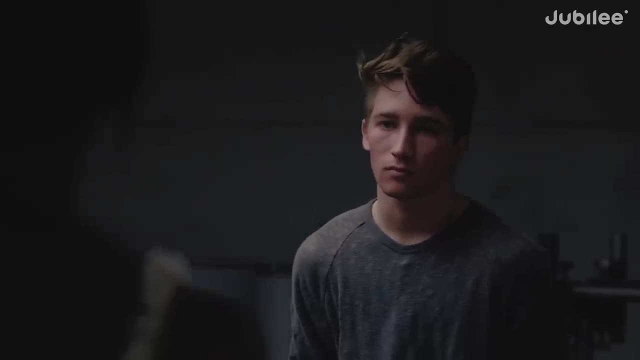 but they never did it, never turned it in and it just dropped my grade completely. Did you tell your teacher? Yeah, She didn't care. Yeah, teachers don't care. She just says you have to talk with each other after school. 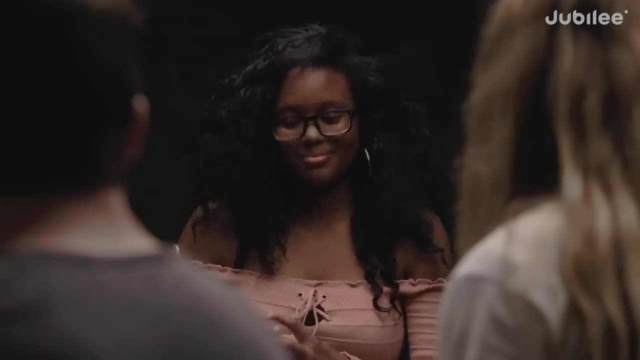 and I do that. Like, can we just all agree that teachers really do like- I don't know how to explain it or put it? Yeah, like the pressure of teachers, Like you can have a really chill, mellow teacher. 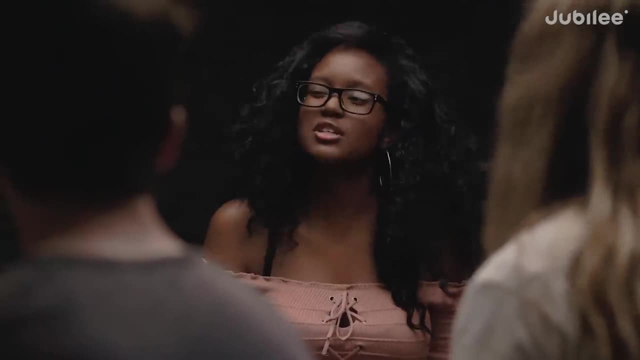 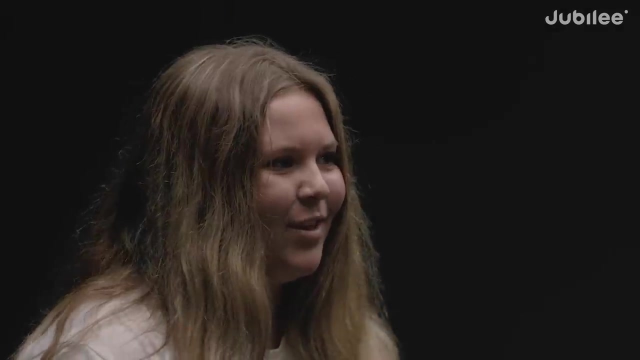 in your worst subject and it'll make you work harder and you can have a really strict teacher in your favorite subject and it will like make you slack. Are you planning on going to college? I, yeah, for sure. 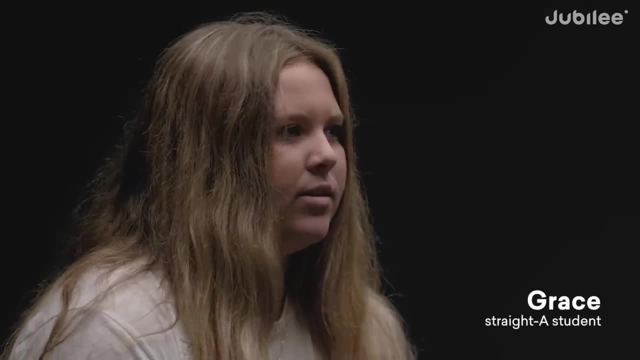 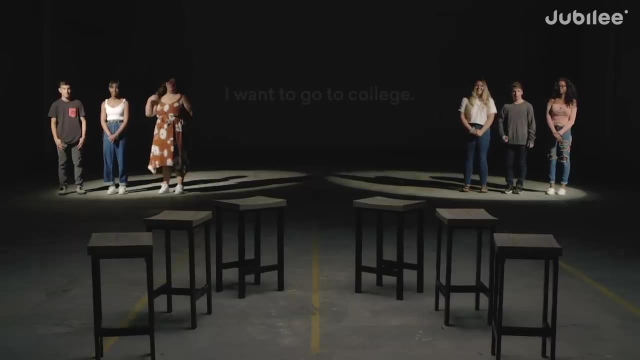 I definitely want to go to college. I think I want to go to law school and go into, like the law profession. I started doing debate last year and I can't solve, so yeah, I want to go to college. Me and my parents haven't really had the confidence to go to college, but I've had the college that I want to go to set on since I was like 10.. But yeah, I want to go to college for me because I want to become a better dancer. 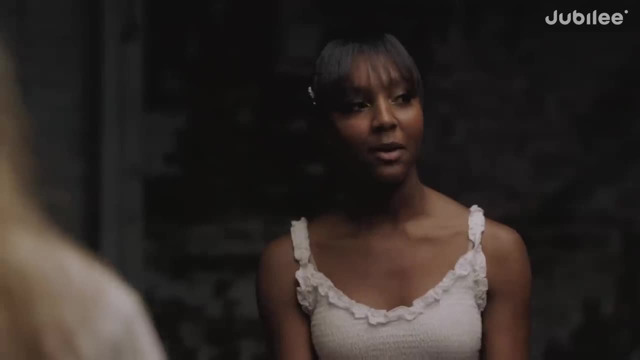 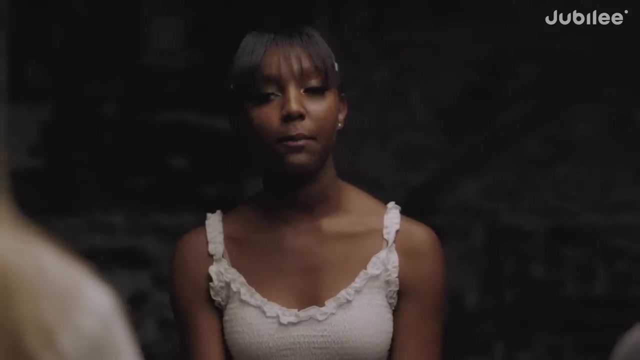 and then I also want to perform and then afterwards make my own dance studio and all that stuff. But I want to be a performer and I can't be the level of performer I want to be without being able to go to college. Yeah, I think I do it. 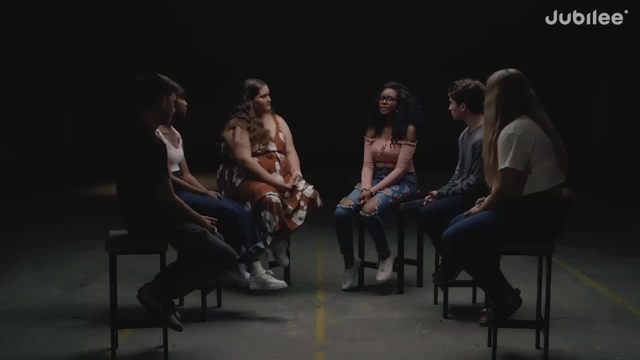 for like another reason too, Like I have to go to college because of my career choice, but at the end of the day, there's kids in countries that get killed for reasons like reading books, that have to travel across rivers. 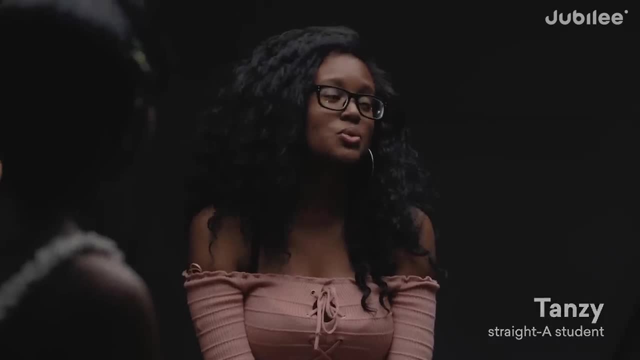 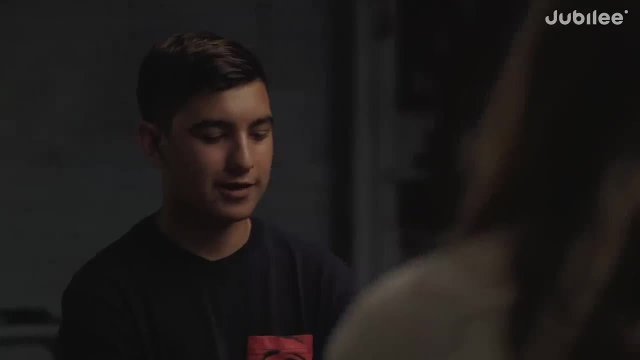 and jungles just to get an education, and I think sometimes we do take that for granted. I want to show that education is very powerful. The wanting like. I don't exactly want to go to, like college, but I want to go to a trade school. 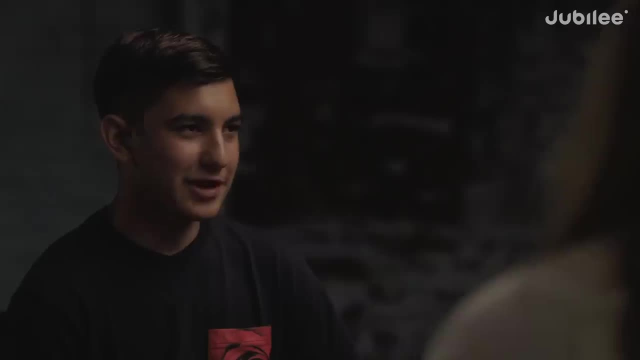 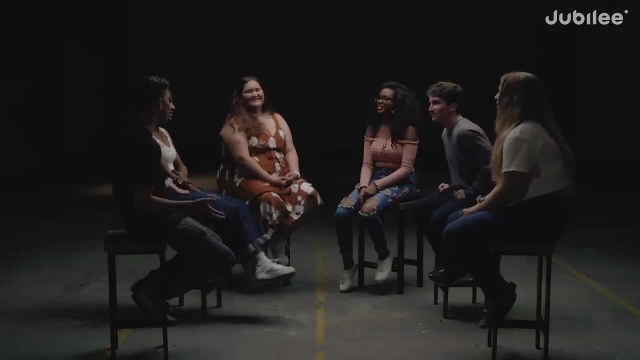 so it's kind of like an after-school, after you know, But it's like I want to go and experience being in a different place, like not being in high school, People coming from all these different places, like it's so like. 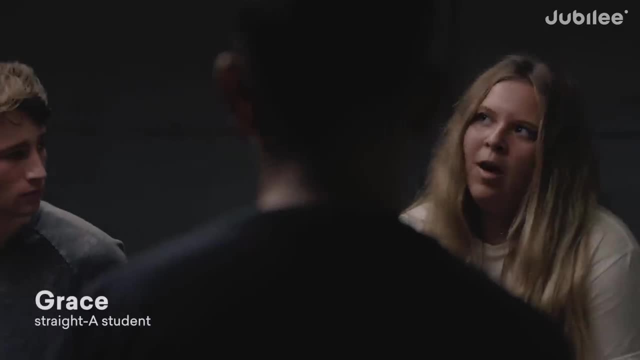 it's so different, Like you know. so I kind of feel like the opposite side of like what you guys are saying. I want to go to college, but the reason why I want to go to college is because I feel like 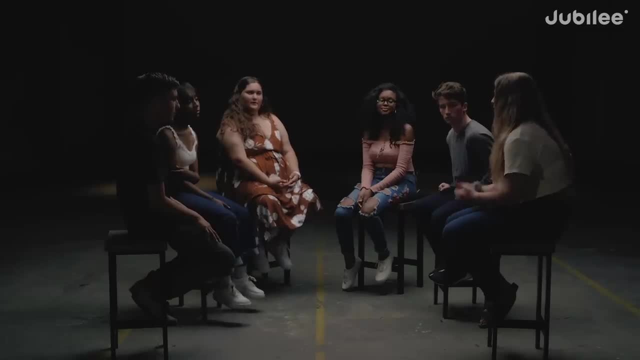 it's the thing that like make me feel the most successful and like it's still like my own desire and my own want. I want to go to college mainly just so I can like make myself a good life. 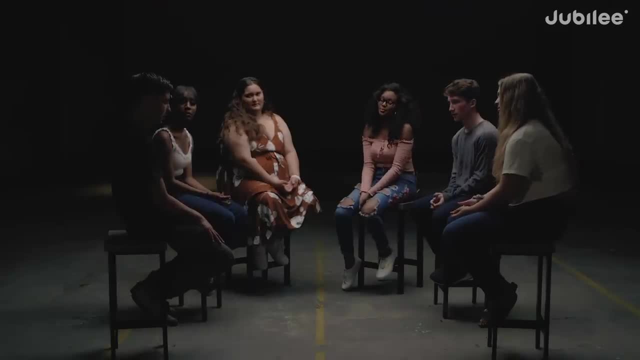 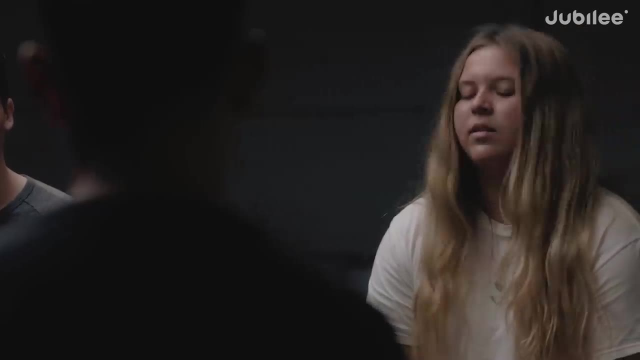 and make myself a good career. Another thing is like don't always like think that because somebody goes to college- like not no offense to you, but like it doesn't always come the way- you think Like just because you go to college. 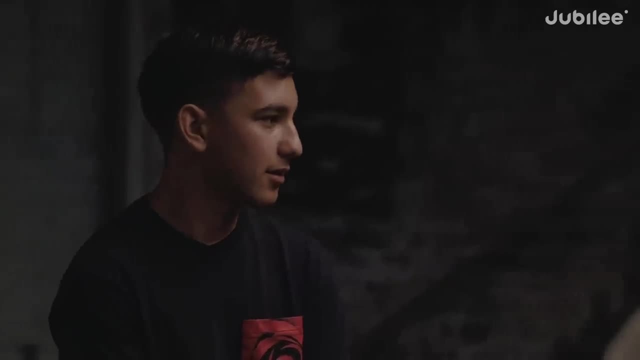 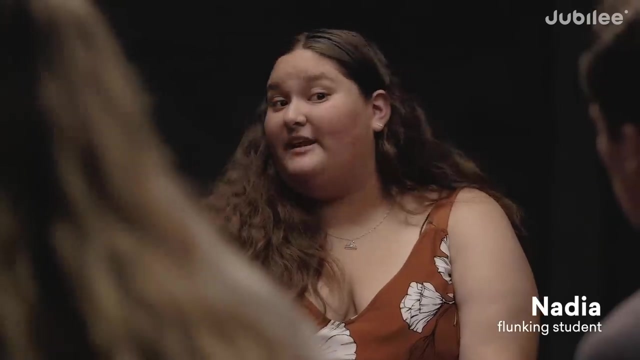 doesn't make you exactly the most successful. I mean, like I want to go to college to make my family proud. I come from a family where, like we're all Hispanic, Not many of us have ever even thought about going to college. 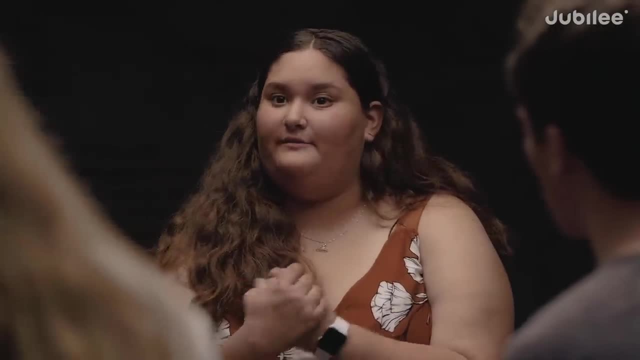 The thought of college, the thought of high school, graduating high school is really like. it's like wait, like you graduated high school, So I'm like I don't want to waste my opportunities. I'm not going to take. 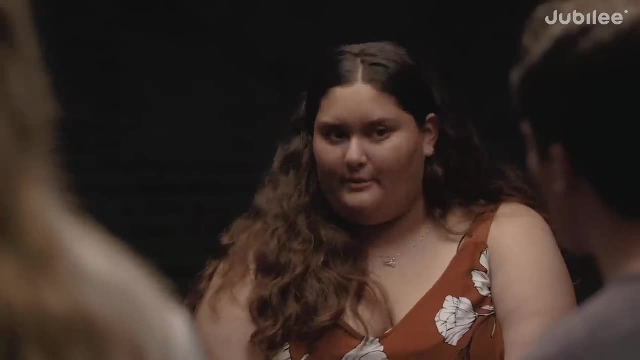 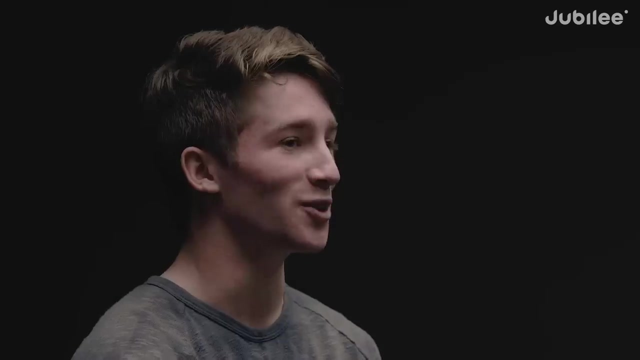 these chances for granted, Like I am going to make myself proud and my family proud. Was it difficult to get straight A's through high school? Hell yeah, I'm not one of those naturally like smart people who can look at a book and instantly know. 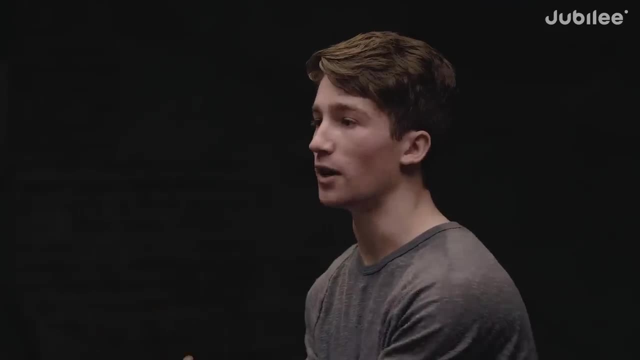 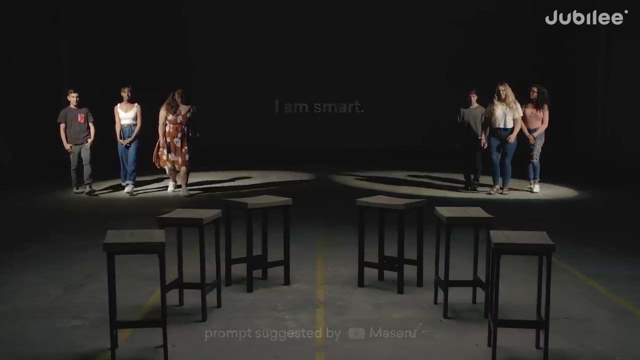 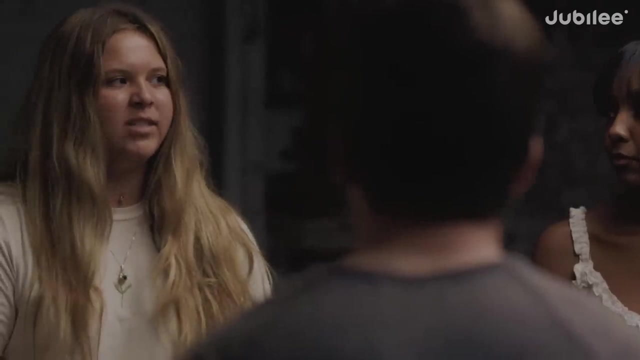 I think our education system is very like: set into these like molds of how you need to fit. Not everyone fits into the mold of a high school. I am smart. There's so many things that define smart, and it's not just being book smart. 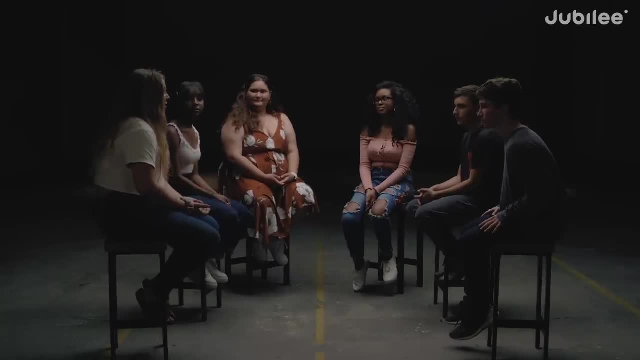 or street smart. It's smart just knowledge, And I have a lot of knowledge and I know a lot of things and I value that knowledge, which I think is really important also to being smart. Yeah, I mean, it's how you use. 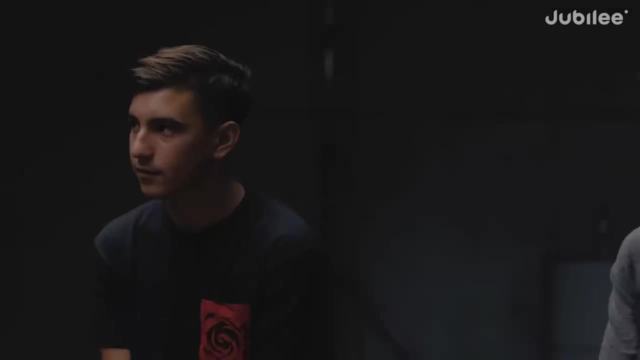 the knowledge that you have. I am smart no matter what Like. just because I'm getting an F on the test doesn't make me dumb. I can be book smart. I'm also street smart, Like I know my way around. 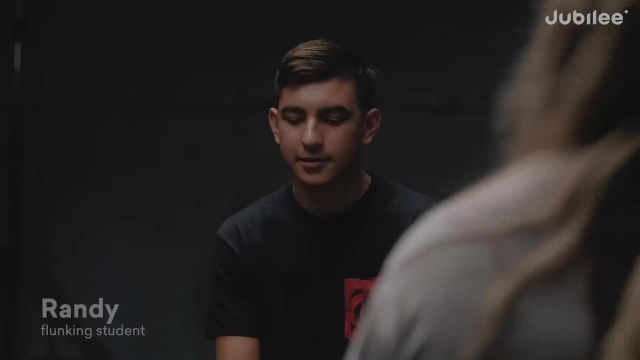 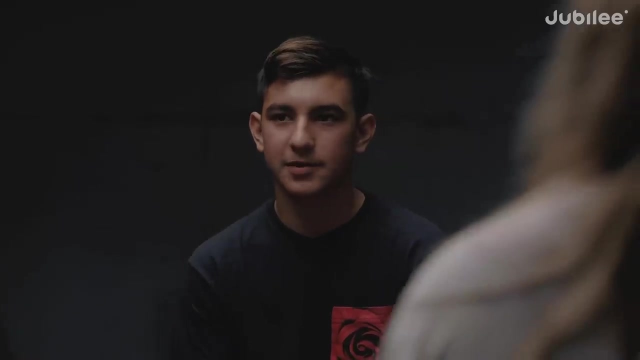 I know my place and I know where I need to be. Yeah, to say you're smart is like something that everybody should be able to say to themselves, Because, no matter what, even if you don't feel like yeah, I'm the smartest person in the room. 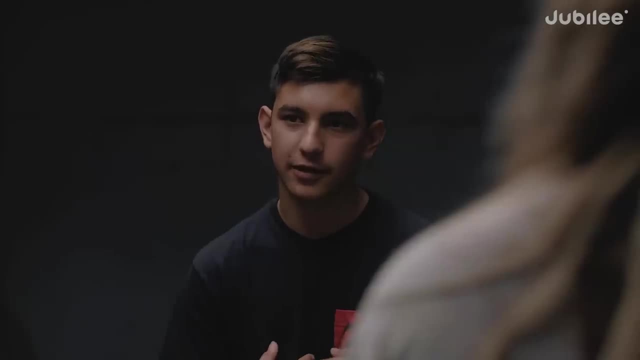 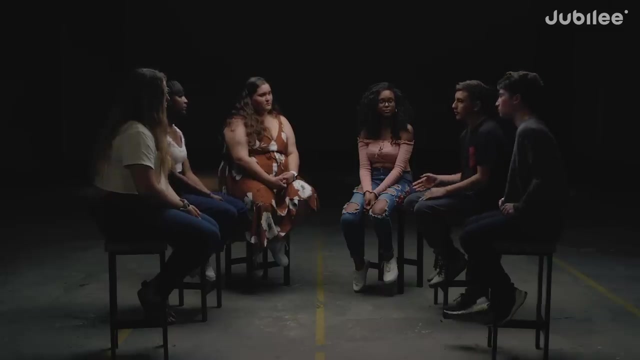 like you might not feel like that, but you're smart to yourself. Like you, you're the one, you're the only person who knows how your body works and how you feel. You're educated on yourself. You're educated on the people around you. 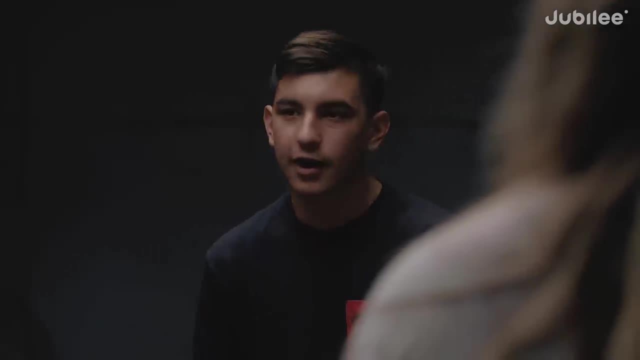 your friends, you know. So it's like you might not know something about her that I know. that doesn't make you like dumb compared to me. Like you know what I mean. Like everybody's still smart in their own way. 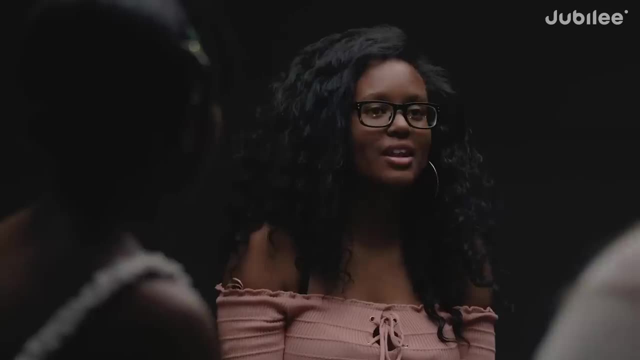 I feel like everybody has something to bring to the table, no matter what, Like. at the end of the day, school's just like the first start of our lives. You know, we're stepping out, we're learning new things. 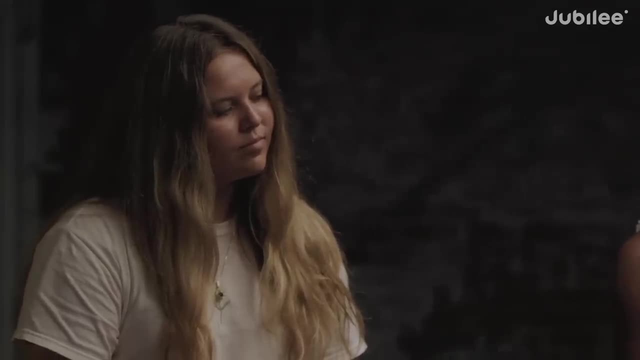 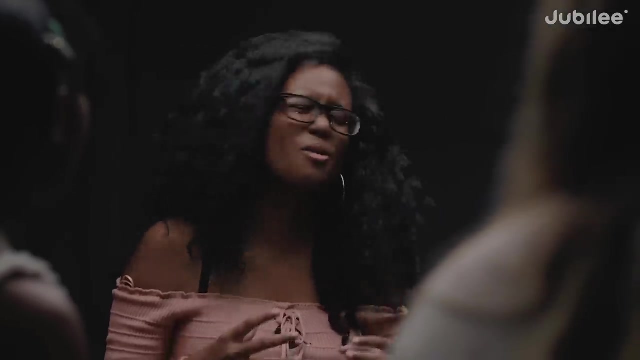 And not to say like grades are like insignificant, but at the end of the day they really shouldn't like put such a hold of you where you like cry or you're depressed or something like that, or it makes you feel dumb, you know. 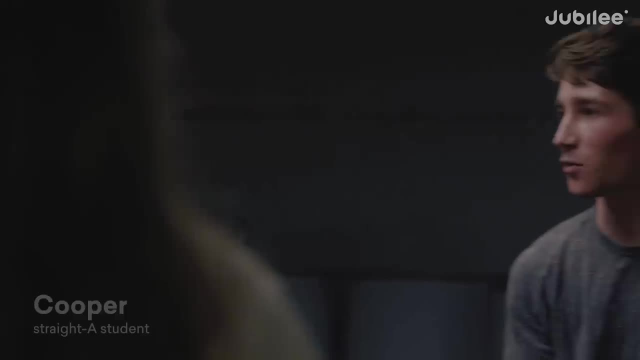 Smart is such a dumb word. It's like: why, like, why do we use it? I think all of you are like so freaking smart. I don't give a shit about it, You know, you're 2.0.. 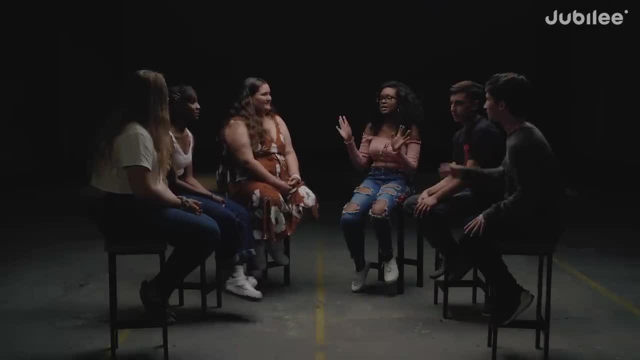 Like I don't care. You know, it's like I think You're bright. You're bright as hell. Yeah, you know, it's like the. It's the person that matters, And I hope that all of us. 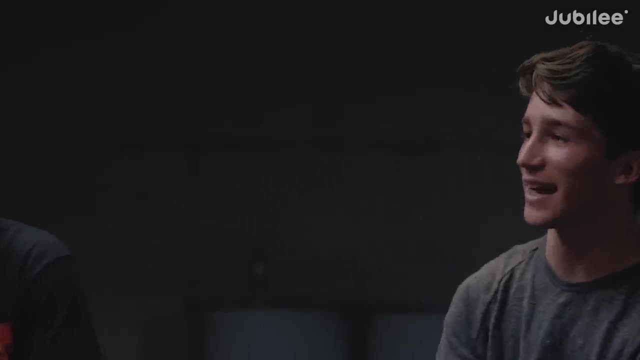 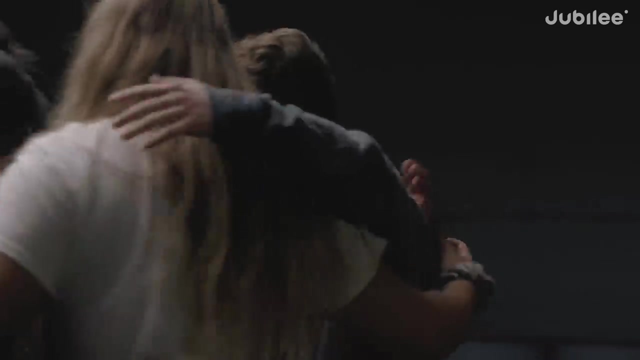 actually know that. you know, because that's what's going to define us in the end. That's what's going to make you successful. Yeah, It's almost like group hug or something. Group hug- Yeah, all right, We're smart. 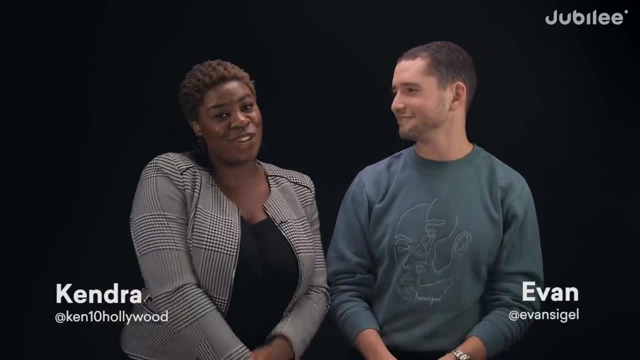 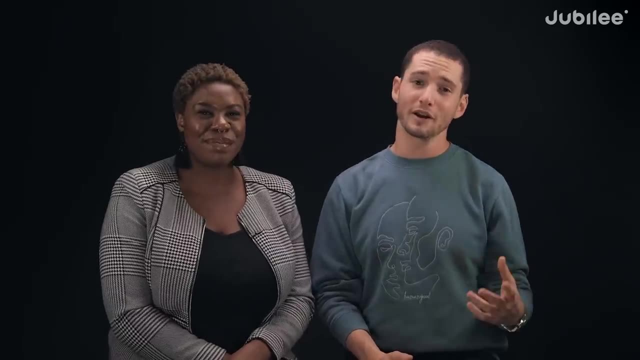 Aw, that was super endearing. I love that episode. See, I was a straight-A student, No comment. This episode dealt a lot with education, the importance of grades and if you want to learn more about education or see what it might look like. 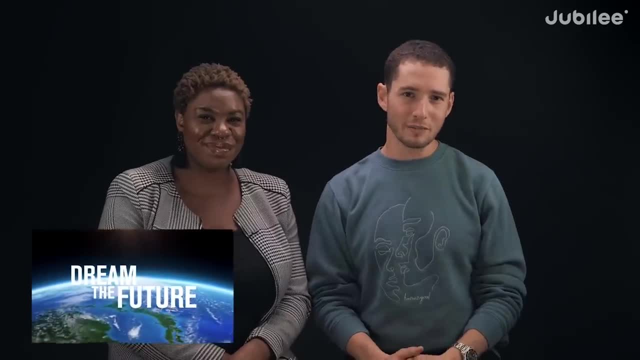 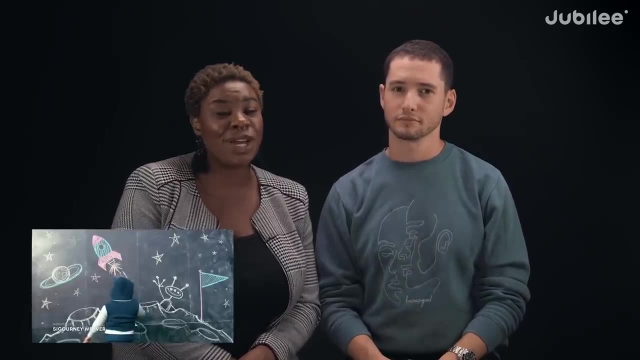 in the future. check out a series on CuriosityStream Dream the Future, specifically an episode called School of the Future. It's narrated by Sigourney Weaver and examines how we might be able to use technology to make learning better for students.